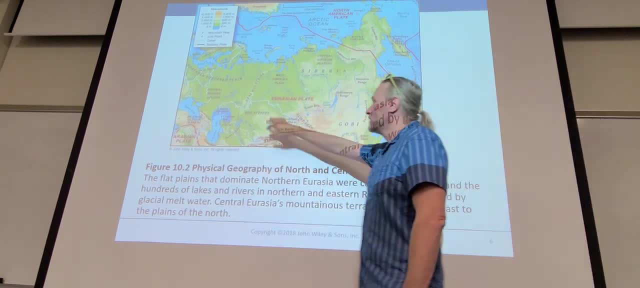 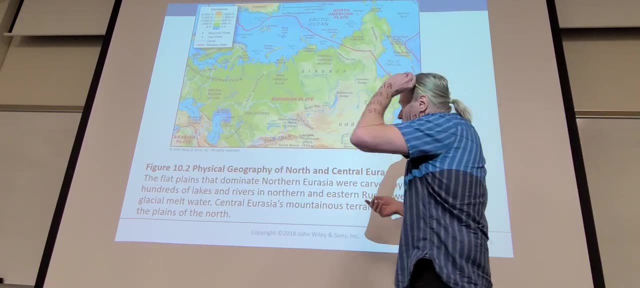 They have. But most the population to this side of Euro Mountains are considered more Siberian populations. But most the population to this side of Euro Mountains are considered more Siberian populations, Siberian populations much less populated over here in the Siberian area for a 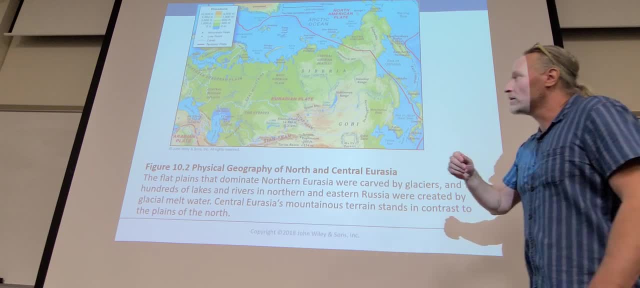 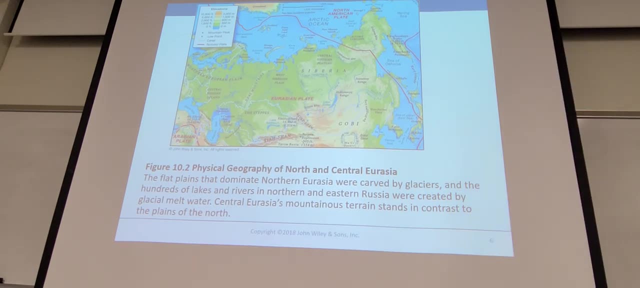 number of different reasons, one of which being, well, it's really cold in all of Russia, right? but you know we live in a cold place. we know you can. you can live in a cold place and make it work. well, this is extremely cold in this area here. 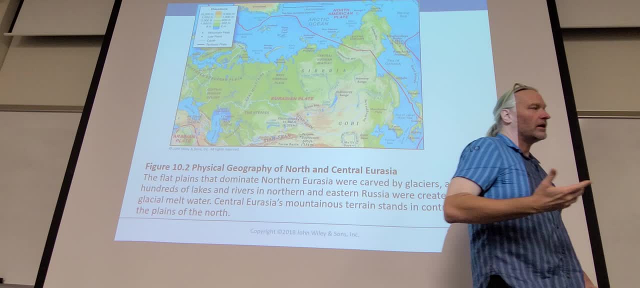 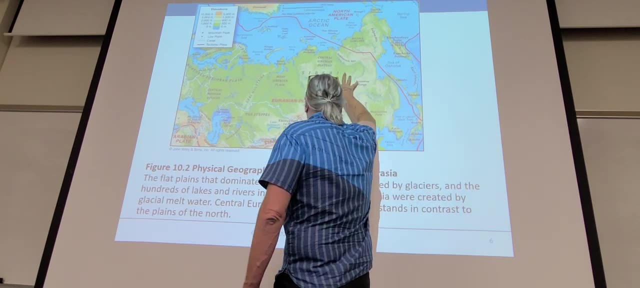 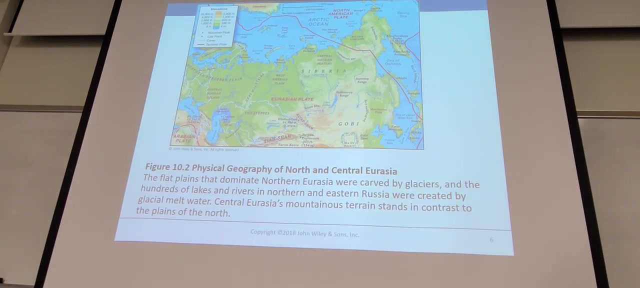 when it's not frozen for half the year, it's all extremely swampy, and so it's just not a great place to live. as you can see, going even further east get higher elevations, so it's even colder. even though this is very far north already, it's even colder on top of that, right, let's see what else about the. 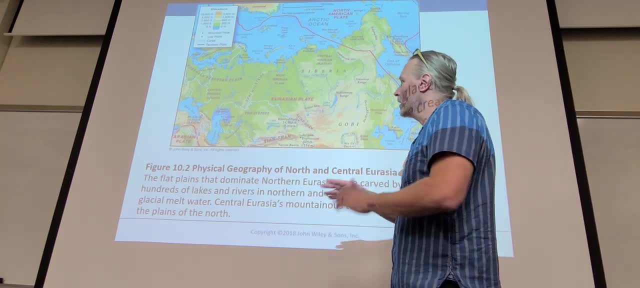 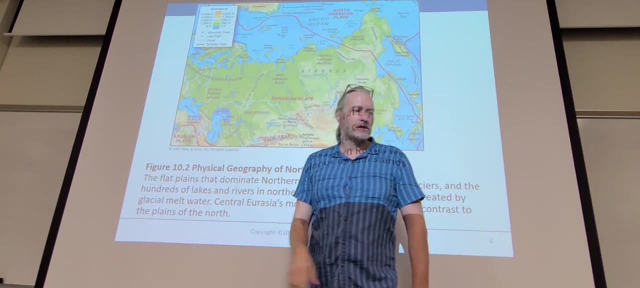 physical geography of the area. well, you'll see areas that are called the steppes. we're also going to look at the RLC here a little bit, the steppes. this is a climate that is it's like step climates that we've looked at elsewhere. it's not. 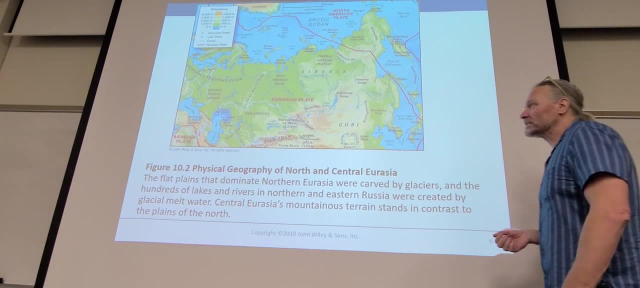 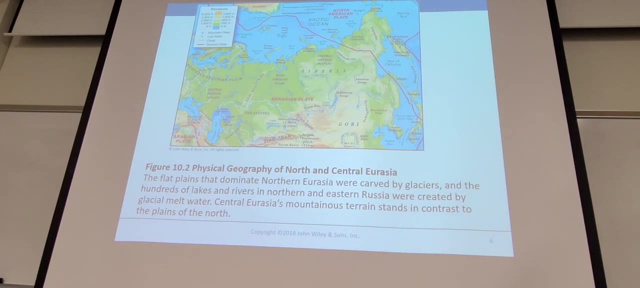 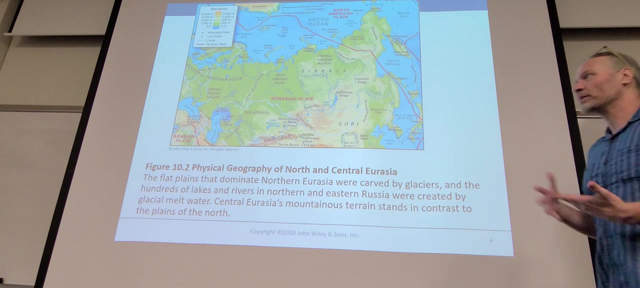 desert but it's pretty darn dry. usually step climates are places where, somewhat like the Dust Bowl in the us, where you can irrigate and get some good crops for a few years, but you got to be careful because there's so much evaporation and 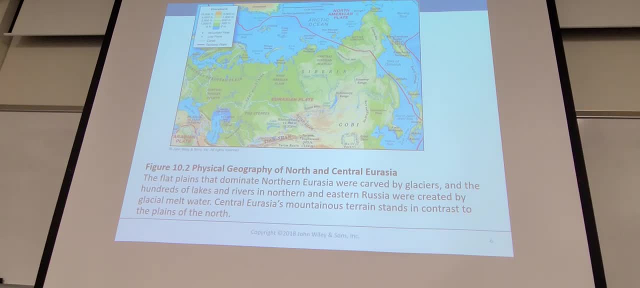 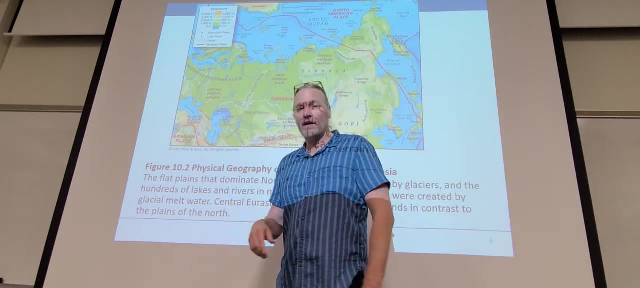 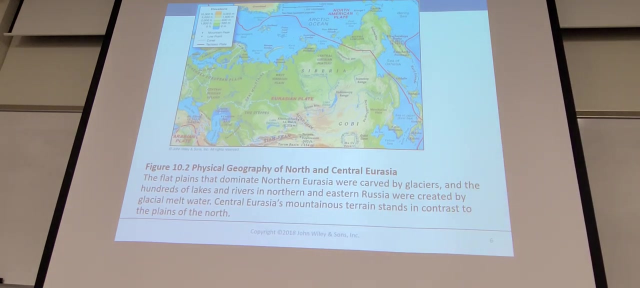 we'll leave behind little particles of salt and you'll get salt build up in the soil through time. this has happened a lot with growing of cotton in the region. lot of areas have been less and less productive, due time because cotton is a very thirsty crop, as they say, Ural Mountains as 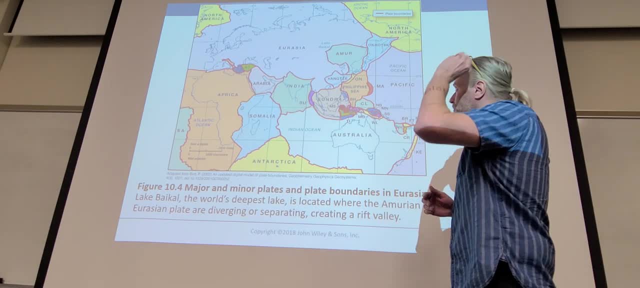 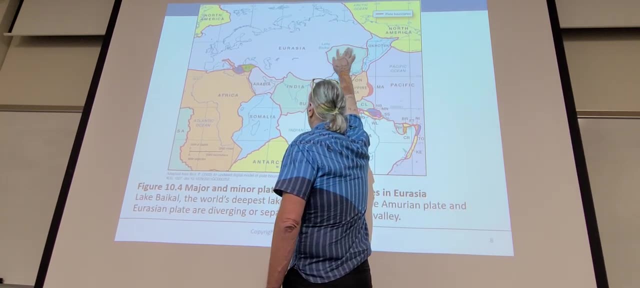 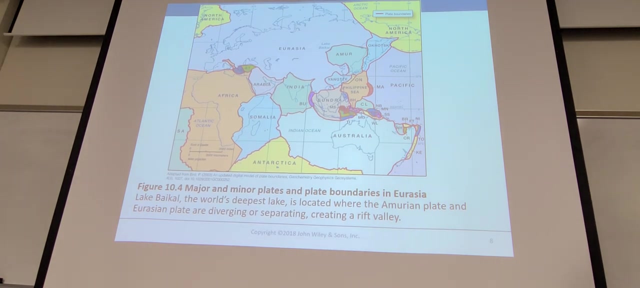 if you see from this map of the different plates, the main plates here is That that encounters this region. It's not a it's very little populated area, but you will see why this lake here is The deepest lake in the world is because you have two plates come together and since it's forcing one under the other, 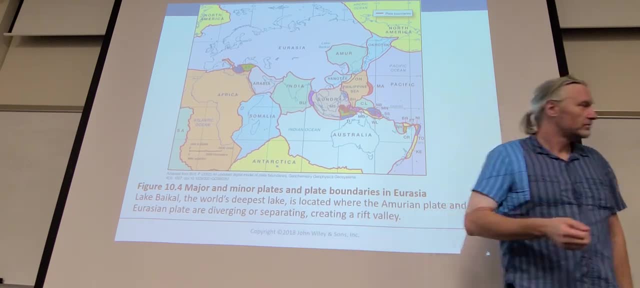 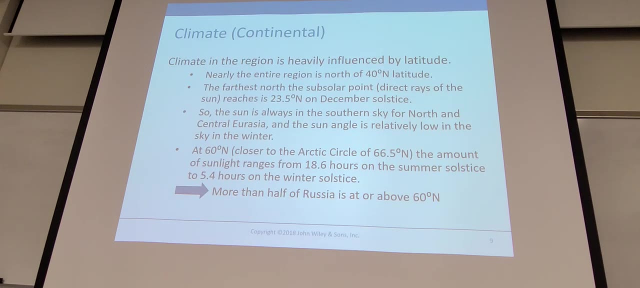 It's creating up a very large gap there. Let's see anything else I can point out. So the climate, the climate in general, is what we call a continental climate. What does that mean? Well, places that are in the center of a continent tend to have more extremes of temperature. 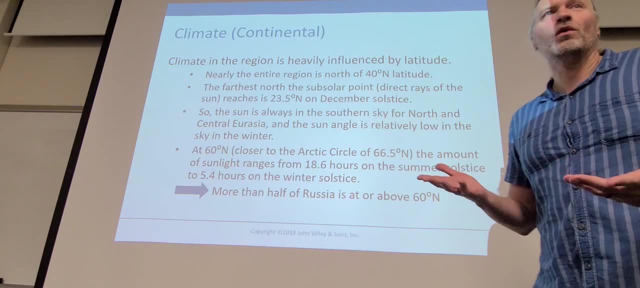 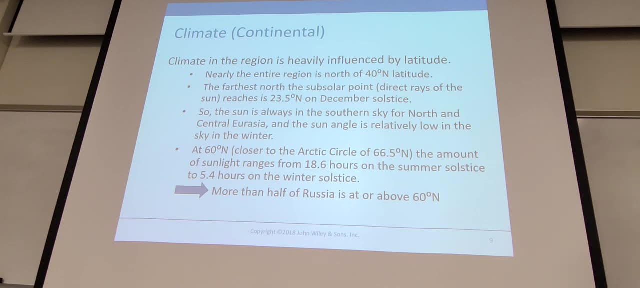 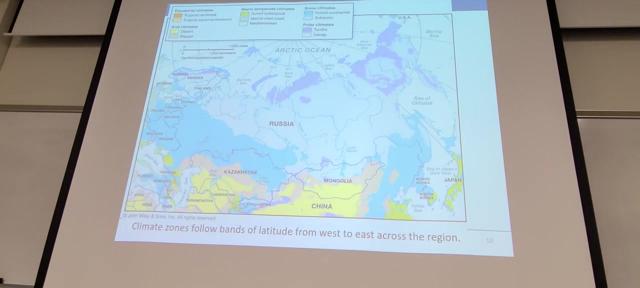 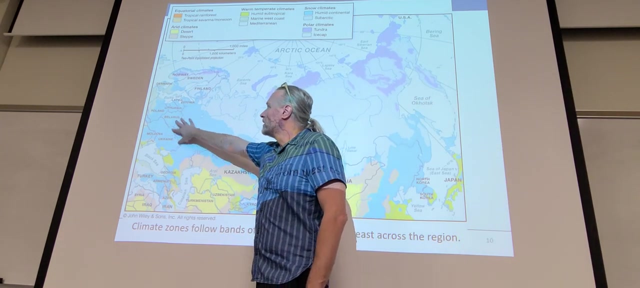 Yearly or even daily, right, and we know that very well here, Because we have extremes of temperature and we're almost at the center of a continent, right, That's the main thing I wanted to say about the overall climate. You can see that well as you move over in this area, right? 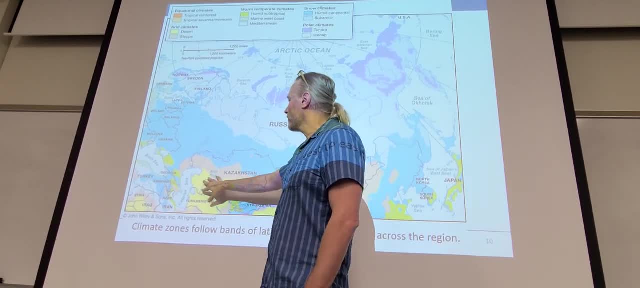 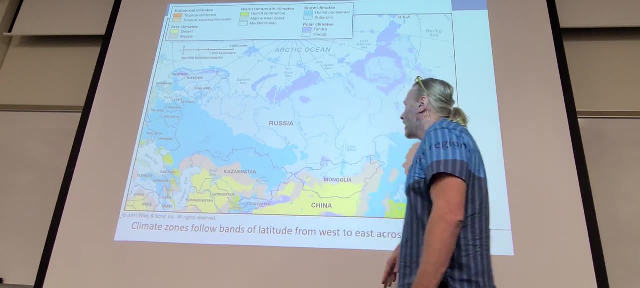 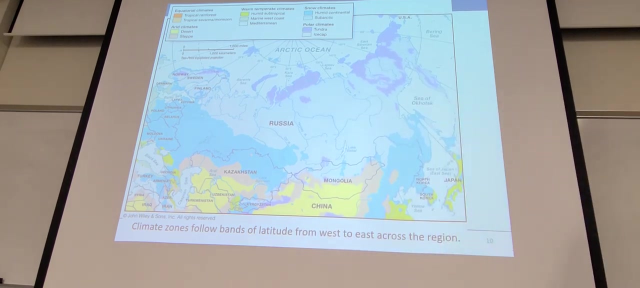 It's still relatively productive. and then when you get further south, you get very different climate regions. right, you get deserts, You get step which is near desert, And then- this is one of the reasons why this area is as I said before- There's very low amount of habitation. 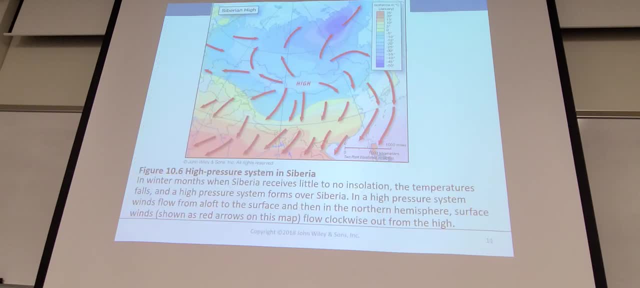 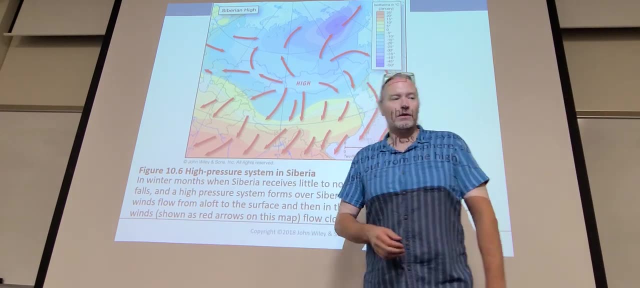 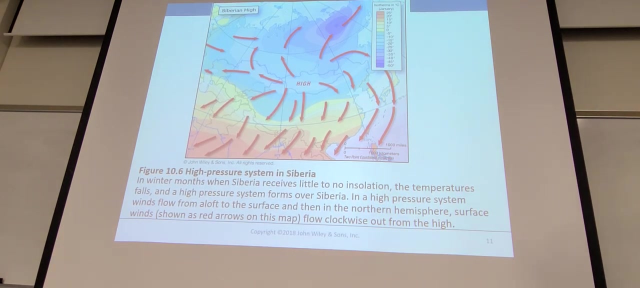 Not a lot of people live in there. The book talks about how there's a constant high pressure system here. high pressure, Well, why would it be high pressure? very cold, cold air falls. right, You know that hot air rises because hot air balloons and stuff. cold air falls because this area is so cold. 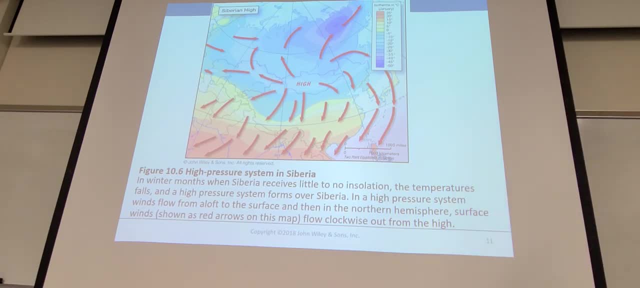 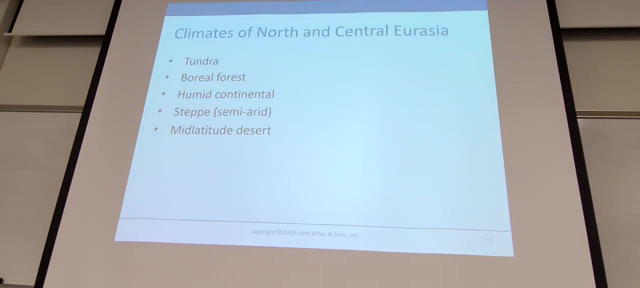 It always has air coming down Out of the atmosphere. when it comes down, it then kind of goes out. in these these ways, the arrows are pointing, But that's what it means when it says it's high pressures. when it comes to climates, well, They're pretty low productivity. 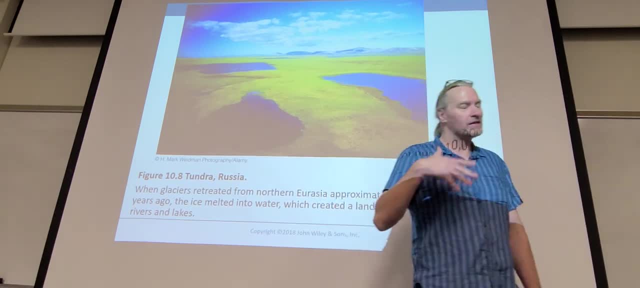 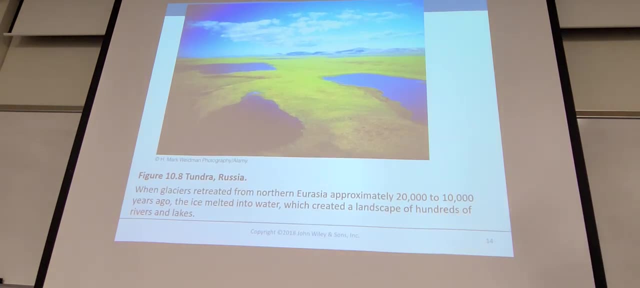 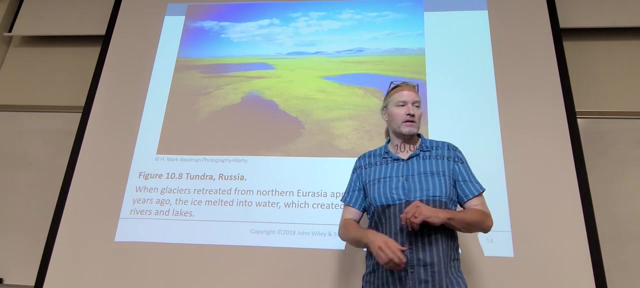 Tundra climates, Tundra- right, it gets a little bit of growth or a couple months out of the year. These are the areas that have actually been in the past couple years. if you read about fires going on in Russia like large-scale fires, Well that is because a lot of these areas are drying out of it. with climate change just a little bit warmer. 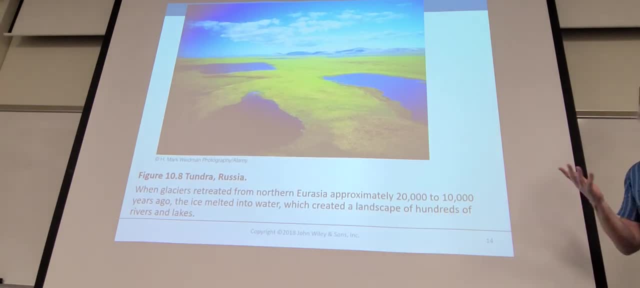 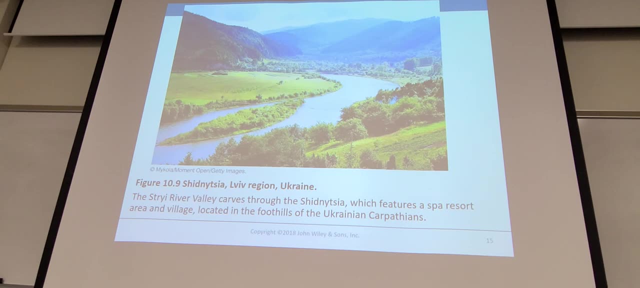 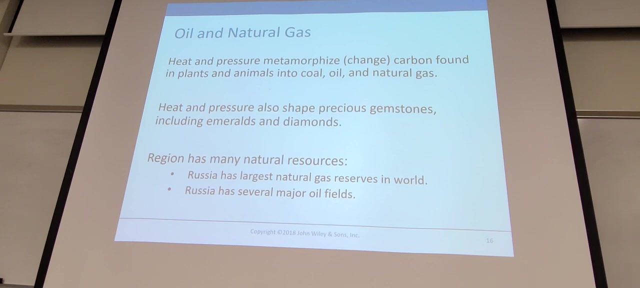 A little bit more time for it to well catch fire randomly. Further south he goes, you can see it's a bit more productive. You can have more agriculture, Oil and natural gas. That's some of the main resources in this region, especially natural gas. It has coal and oil as well. 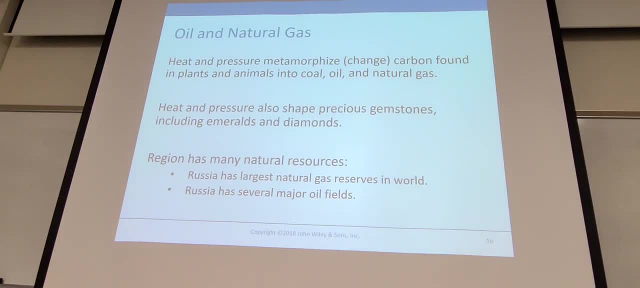 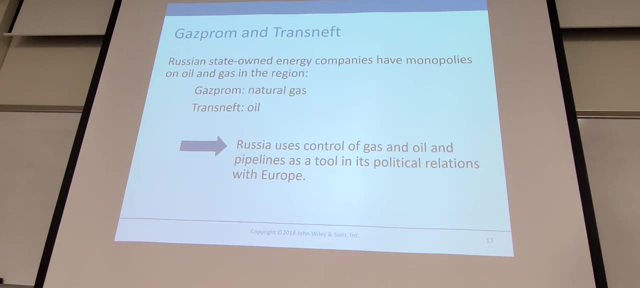 But natural gas is kind of the big source of fuel and in power for Russia itself. so Russia, Their national, the natural gas Company, is nationalized. what that means is the money that that company makes Is there for the country to use for whatever it wants to do. 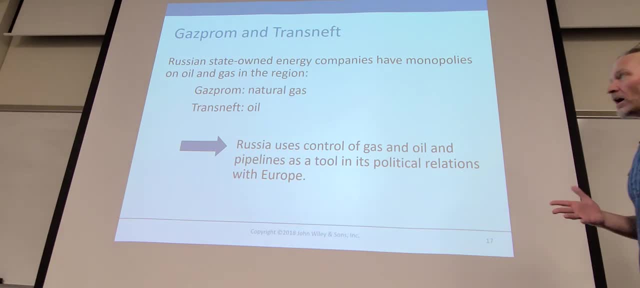 A lot of countries do that still nationalize our resource. But this is one of the reasons why Russia is so vulnerable to ups and downs of fossil fuel prices. if the prices go down, then all of a sudden the government doesn't have money for its own budget, right, doesn't have money for kind of normal. 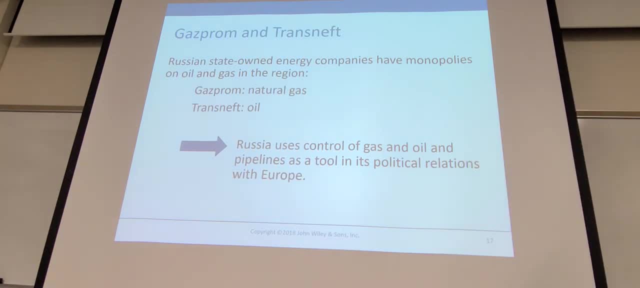 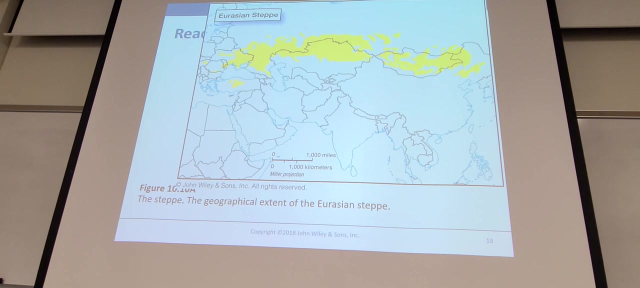 stuff. in general that hasn't happened too much but as I'm sure you all remember, of course the fuel did go down quite a bit at the beginning of the pandemic. Russia was one of many countries that was kind of hard hit with that economically Steppe climate. as I said, these are areas that tend to be. 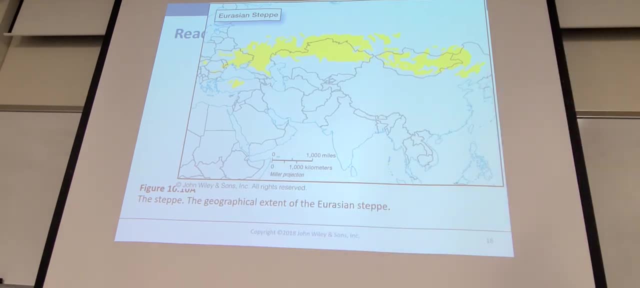 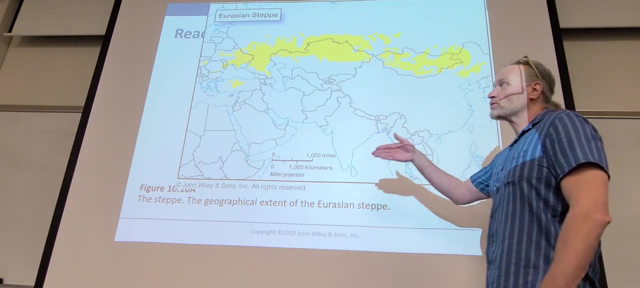 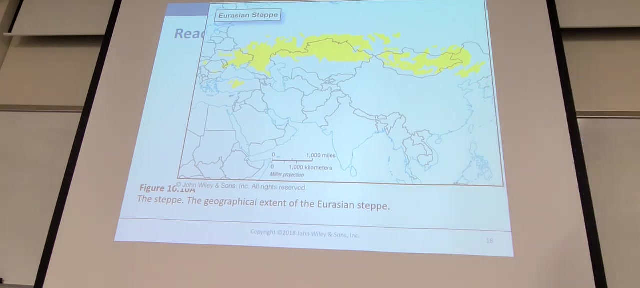 dry, you have some agriculture, but very often the over utilization of the soils in these climates. well, this is one of the reasons why, when we look at ancient societies in different places that have had to kind of uproot and leave because they have overextended their resources, often it's in steppe climate. 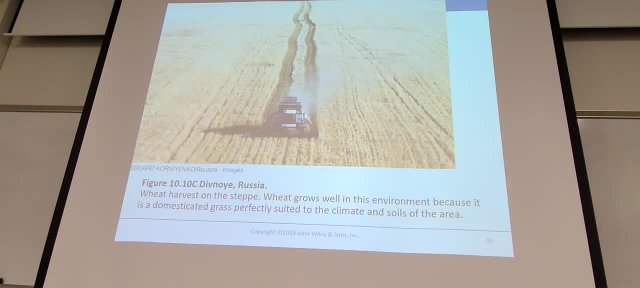 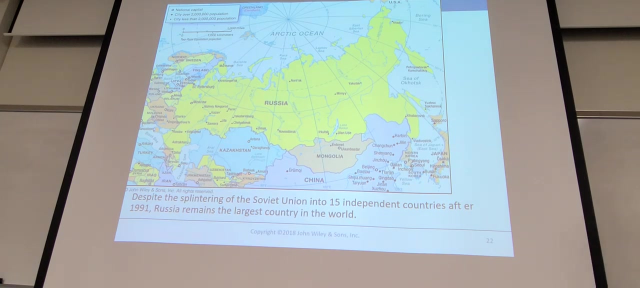 So now I'm going to show you what is the process of steppe climate examples. But as I said, if you irrigate you can get a good amount of crops for an amount of time. Let's see political map. What else can I point out about the political map? When Japan was, 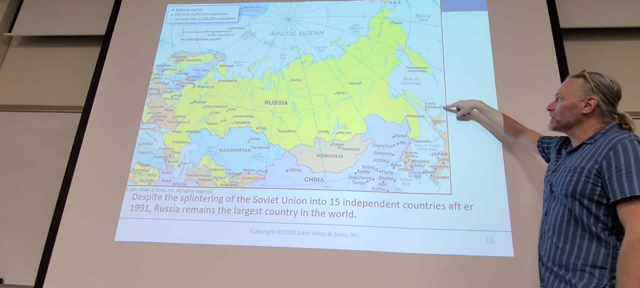 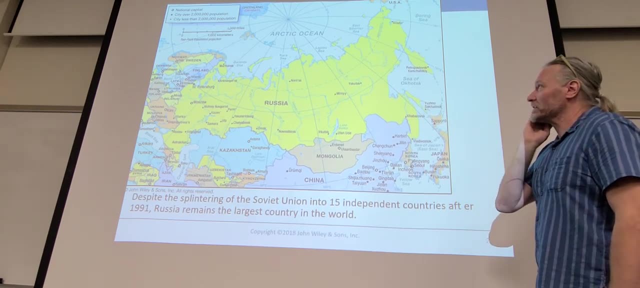 kind of at their peak in the 80s. they tried to buy it back- a number of these islands that Russia basically just took at the end of the Second World War. but Russia didn't really want to sell any. Russia felt like they had really lost. 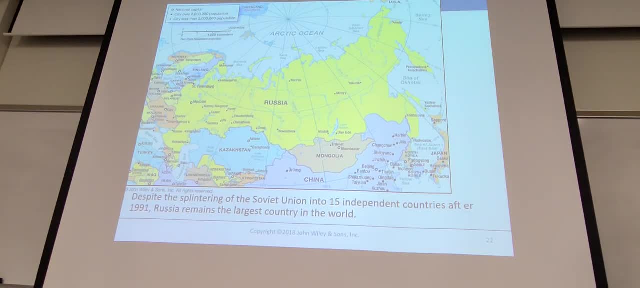 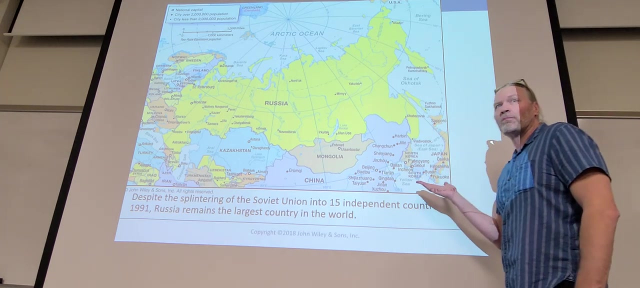 out when they sold the US Alaska, and so they don't want to take any risks of repeated that kind of thing. One other thing I'll point out, since this map is up here, when we've looked at other empires and how they. 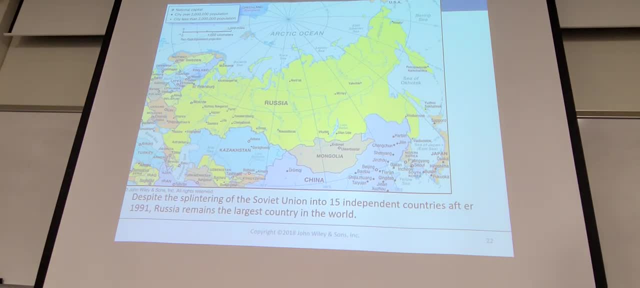 have divided countries up in different ways, those empires. well, when we were studying colonialism, right, Spain or Britain would split places up, not in ways that made sense, but mostly to try to split up different people. so there wouldn't be opposition. The Soviet Union did not do that. What they did was they: 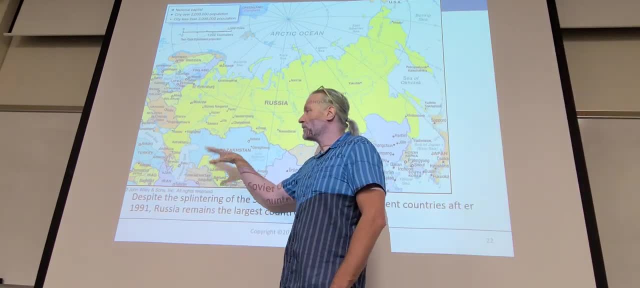 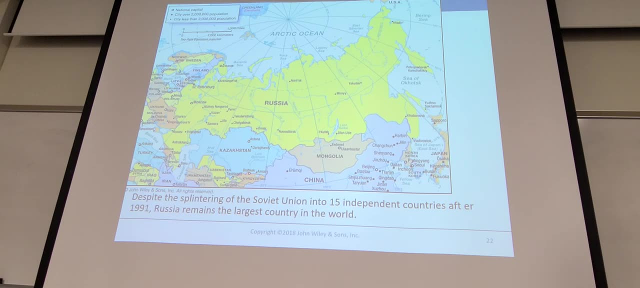 said: well, let's look at what language people speak in different areas and then we'll decide the nation's border. So they split up the national borders based on those languages. It's actually like a pretty reasonable way to split up, to make national borders by language. I 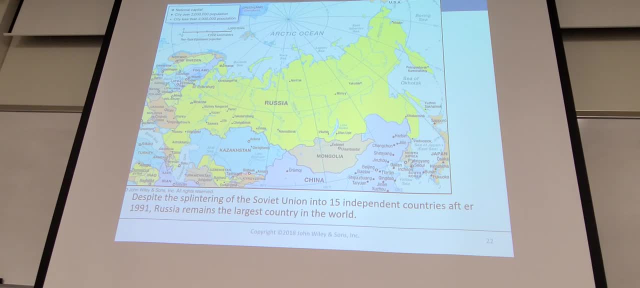 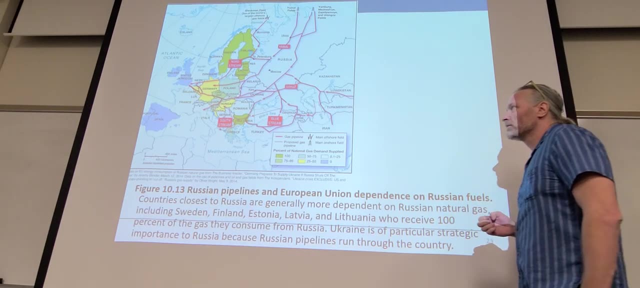 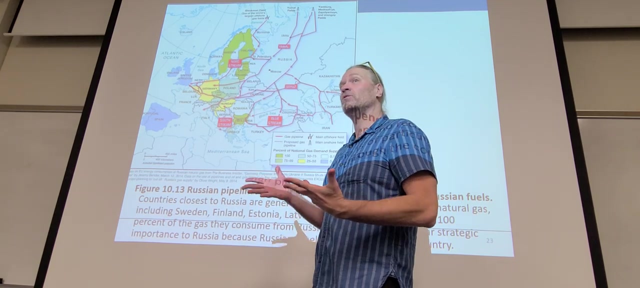 would say the national borders of the rest of the world would look a lot different if that's how they had been divided up. So, natural gas pipelines: Well, if you remember when we talked about all the kind of trouble that's happened with Ukraine and it's in the news again, these, 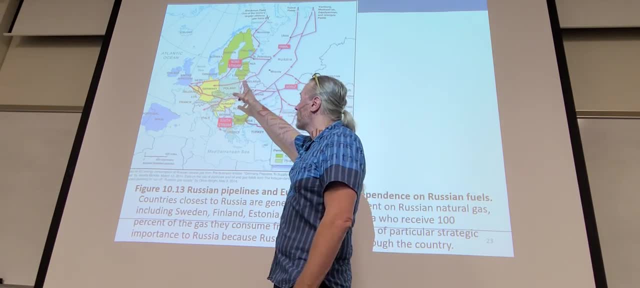 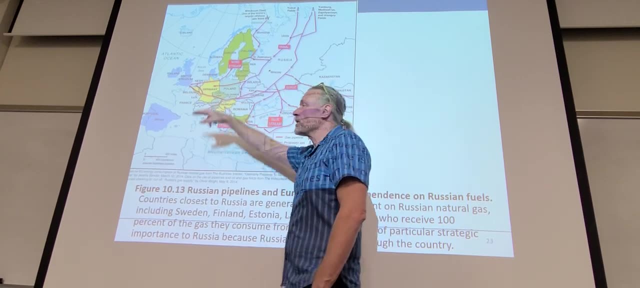 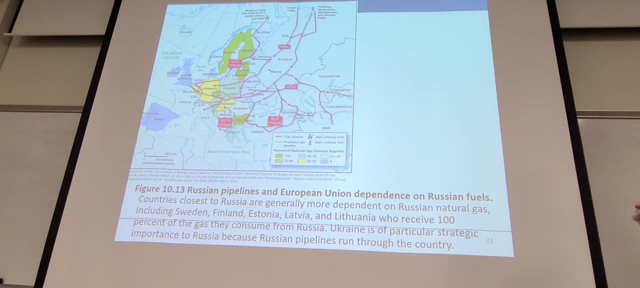 days. part of the reason why Russia wants to have really good control over Belarus, for example, as well as Ukraine, is because they had their pipelines going through them right. They don't want these countries to suddenly threaten to cut off their pipelines from the rest of Europe, where they're making lots of money. 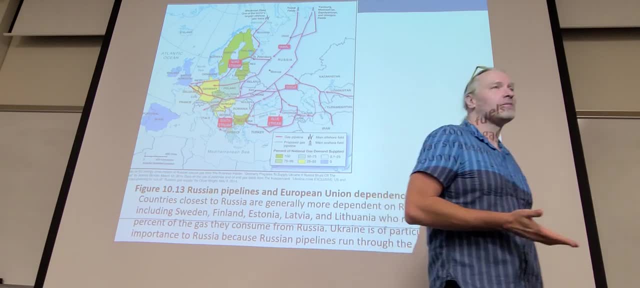 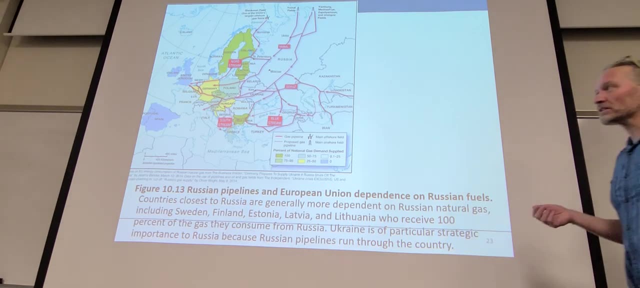 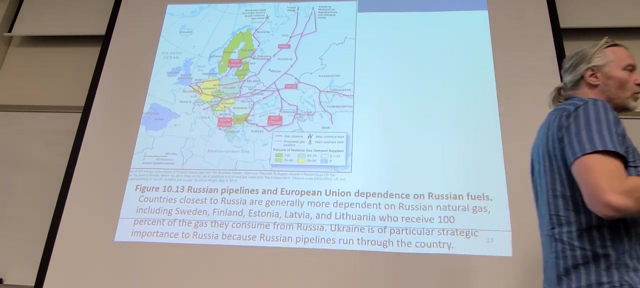 Not that they have anything against cutting off supplies, sometimes themselves. They do do this periodically. if there's something that a different country has done that they dislike, they will just cut off the natural gas supplies. Since Russia has been kind of doing that, more and more Europe has tried to pivot away from using 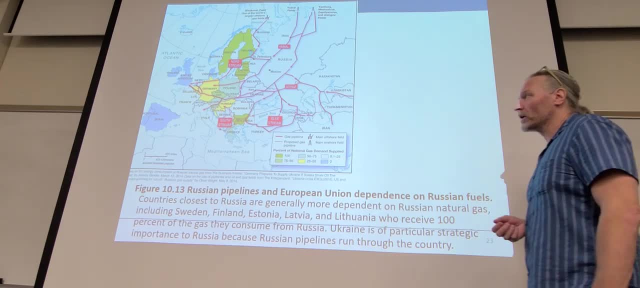 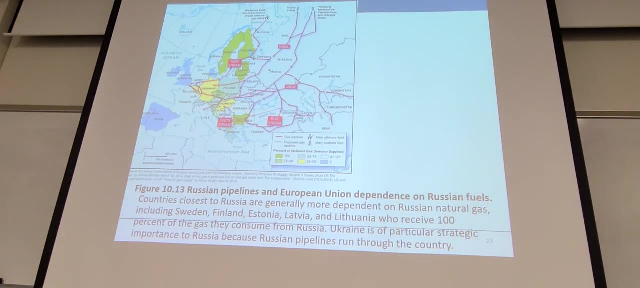 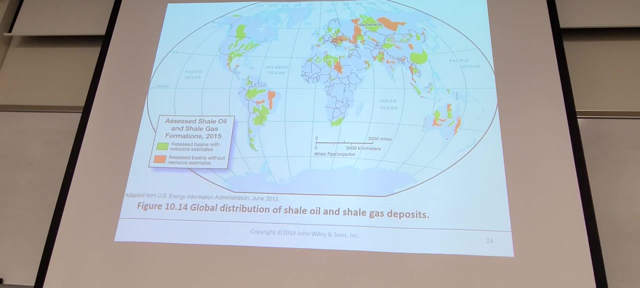 their natural gas as much so they wouldn't be as vulnerable to that kind of thing. Shale oil: Do people know what the difference between shale oil and normal oil is? People heard of shale oil. What's that Shale oil is? 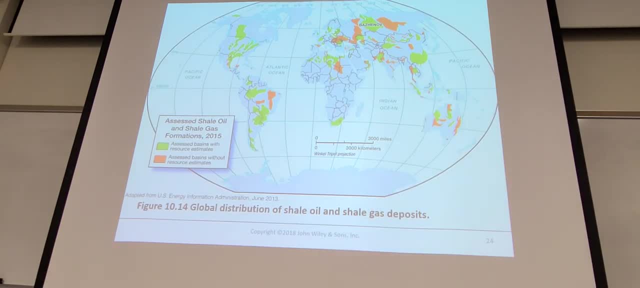 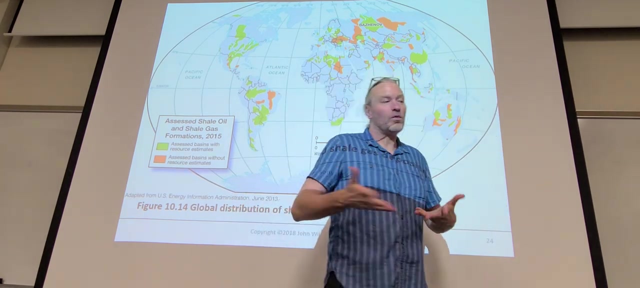 Sometimes oil is found in soil that is really, really sandy, So it's difficult to try to get the oil separated from the sand. It's an expensive process. You've got to heat it up and do all this stuff, So there's actually, technically, there's- a lot more oil in the world than we really 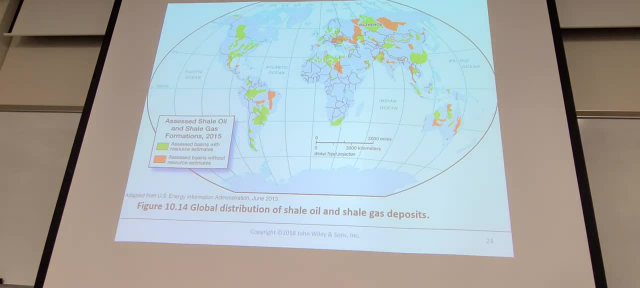 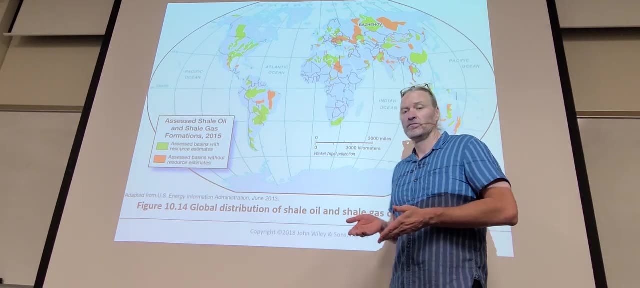 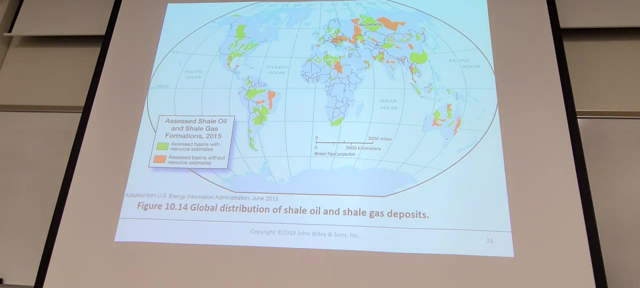 kind of measure. in our normal ways we measure how much oil there is, But shale oil only becomes a thing that is used if the price of oil goes up past a certain amount, because otherwise it's just too expensive. But it's brought up in this chapter because, well, although Russia has a lot of natural gas, 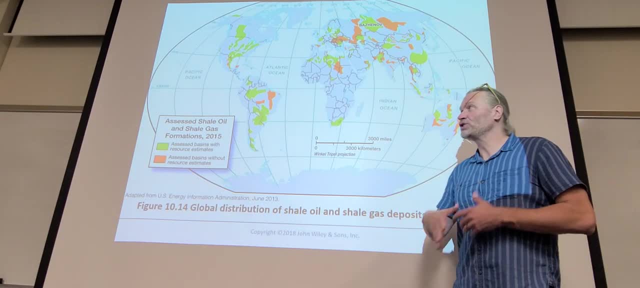 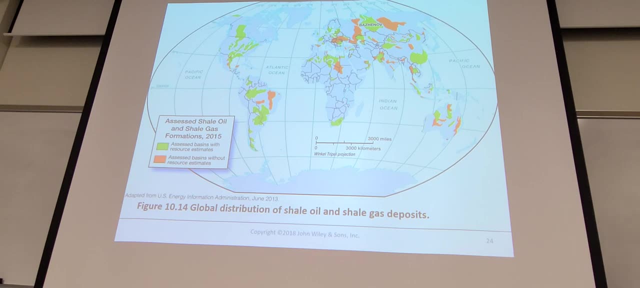 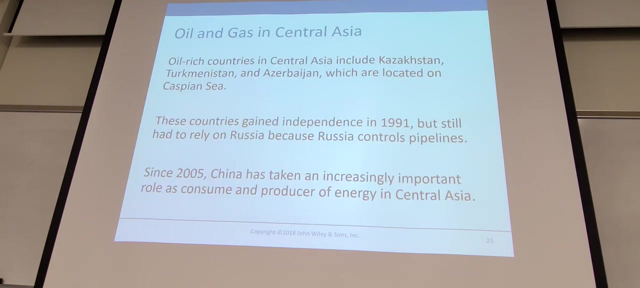 some oil. they have lots of possible shale oil areas that could be large resources in like 10,, 20,, 30 years in the future. Kind of depends on how much people go back to dry them. Let's see here. Oh, one other interesting thing. 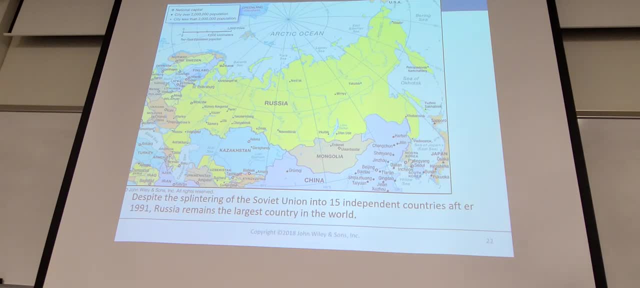 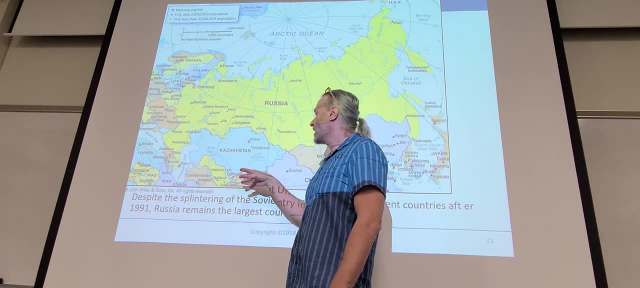 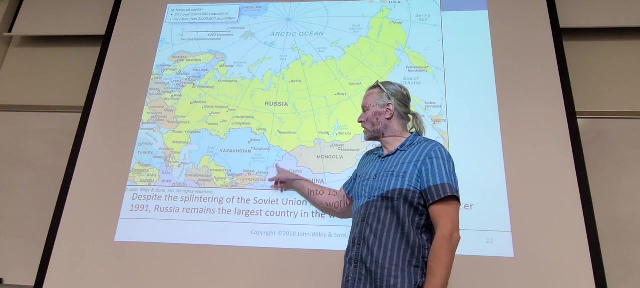 If I go back to the national map, A number of countries especially over in this region, in the former Soviet republics- well, they have more regular oil supplies And you can see China here right shares a border with them. 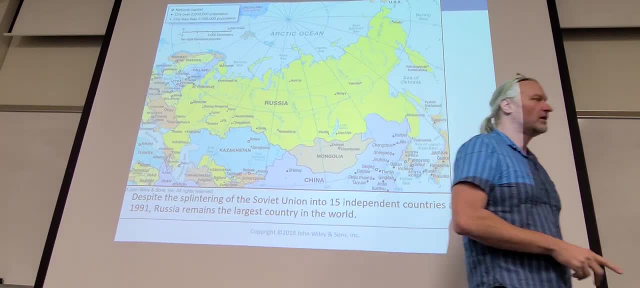 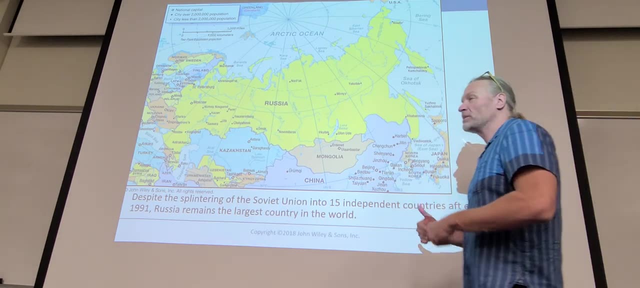 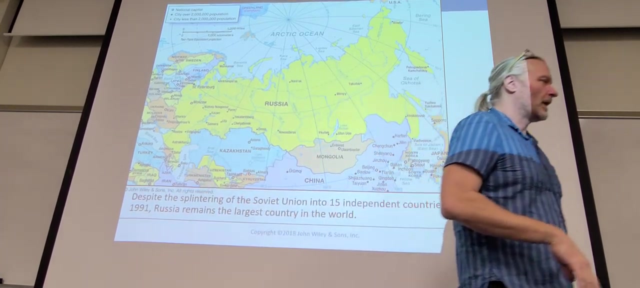 So China has started going directly to these countries to buy their oil, Competing with. usually under the Soviet system, and even after the Soviet Union fell, these countries had certain contracts to give all their oil To Russia, basically for very cheap prices. 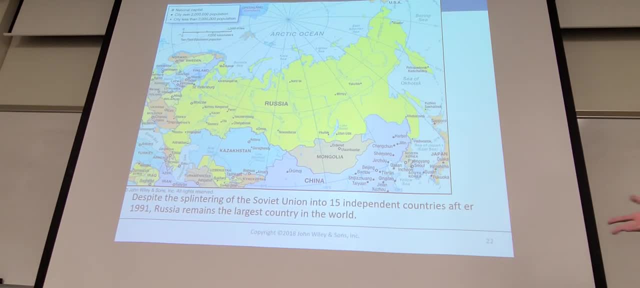 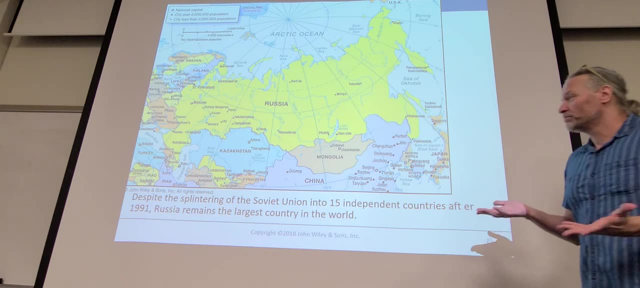 Russia has now been a big fan that China is competing with it in this way. This has led to some amount of tension and hostility, Although it's perfectly logical because you know these countries are just. they're right there, right. 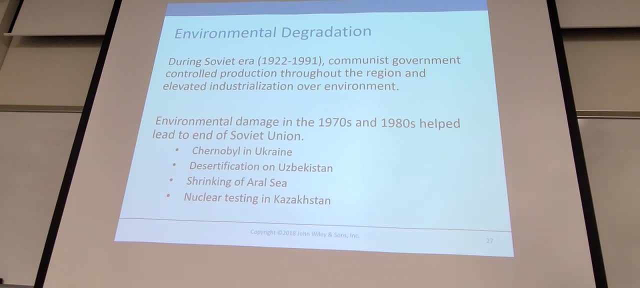 Environmental degradation. So, when it comes to environmental laws, you probably already in general, know that it's been difficult to get a lot of environmental laws passed in lots of countries, right Like the US. there's still people who are pushing for different environmental laws. 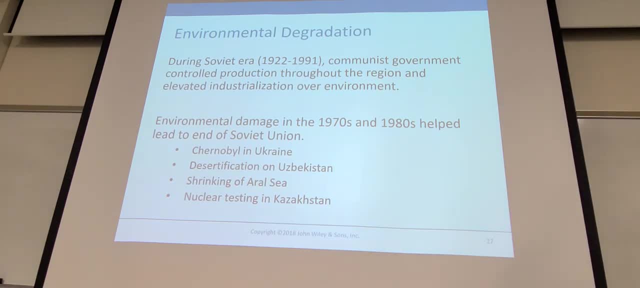 But there are still laws in place. Some of the first environmental laws that happened were just people suing for lower property values. If you have a company that locates right next to you that is polluting with noxious gas, people would start suing. 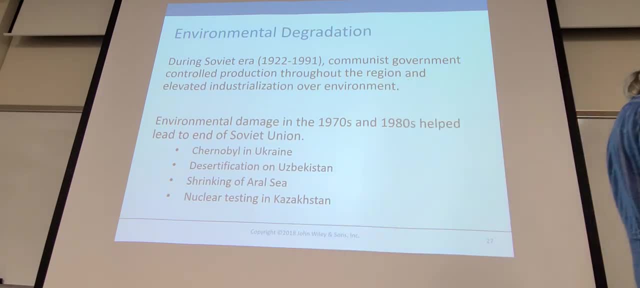 And so slowly. different environmental laws did come into play, Not really strong ones, but like more than zero In the Soviet Union and communist countries in general. there was no recourse for that. Not only was there no real recourse for that, you couldn't sue. 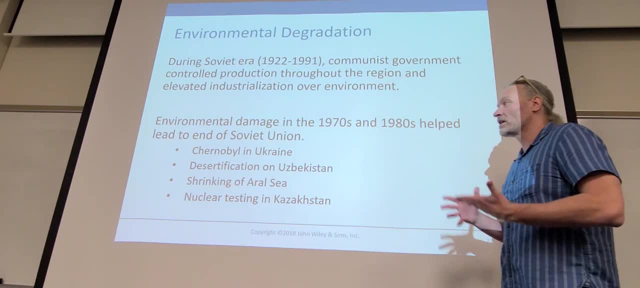 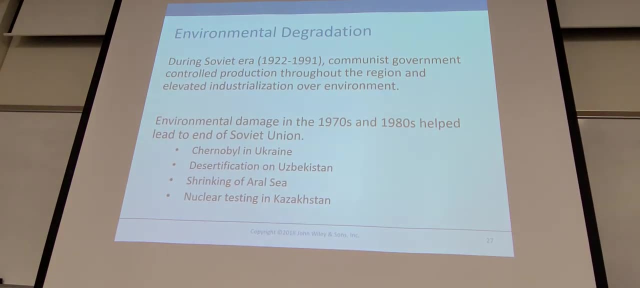 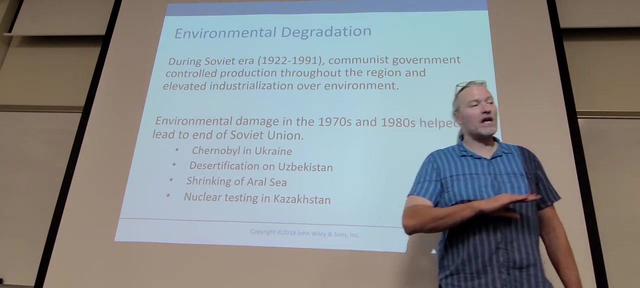 because who would you be suing? The government? The government wouldn't let you do that. The government wanted to push to modernize right So quickly and thoroughly that they really did not look at environmental concerns at all. So you have a lot of pollution in a lot of places. 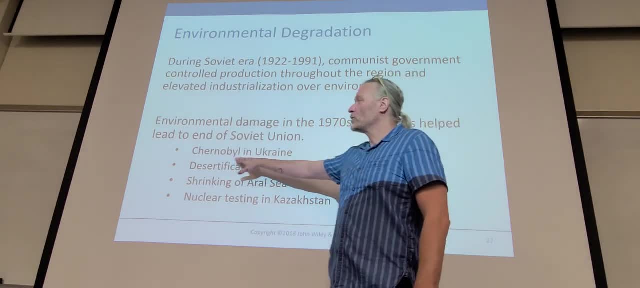 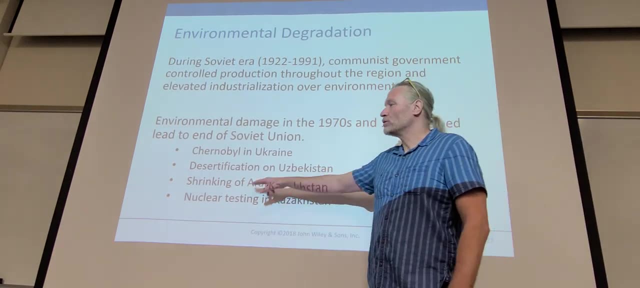 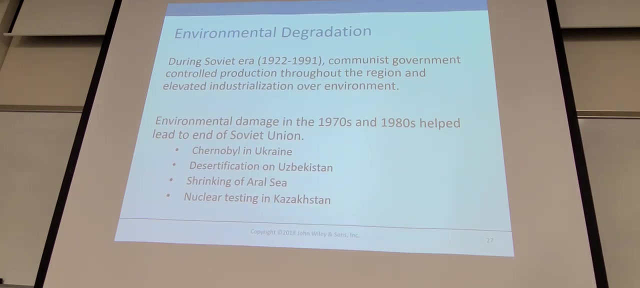 One of the big examples: Chernobyl in Ukraine, A nuclear power plant that went into meltdown. We talked about that last chapter: Desertification in Uzbekistan. Basically because the people who were in charge, based in central Moscow, really didn't care about sustainability of people in Uzbekistan. 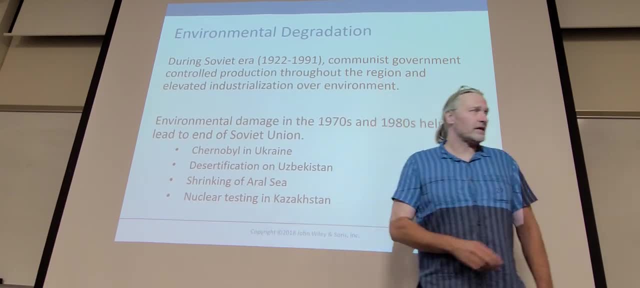 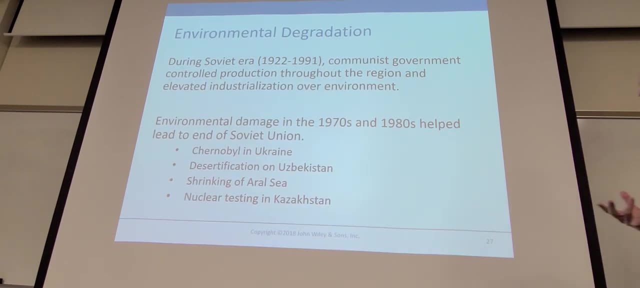 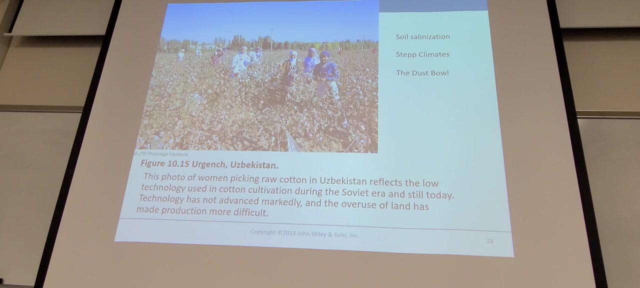 Alright, RLC. similar thing: Nuclear testing in Kazakhstan. Again, it's because the people who were making the decisions were out of Moscow And they just didn't consider the people in Kazakhstan as important. Some of the cotton harvesting The RLC. 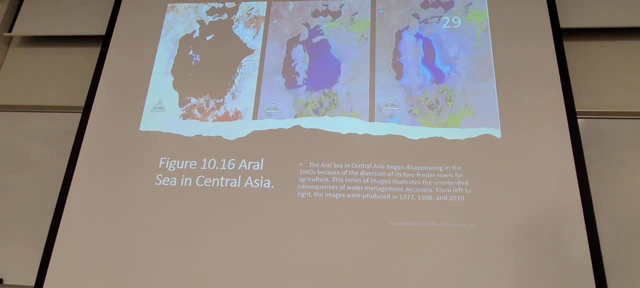 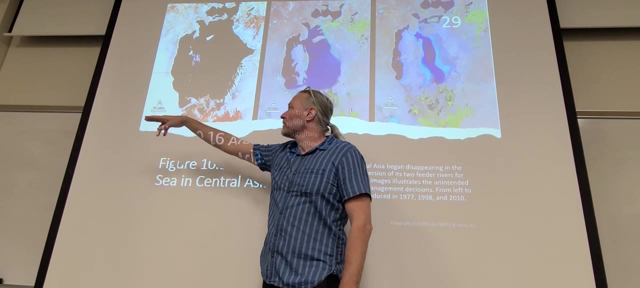 This is kind of one of those classic cases that is in lots of books, especially about climate. But in a nutshell, as you can see, it's a pretty dry area. right, This is red. It's supposed to be green. This is just a false color. 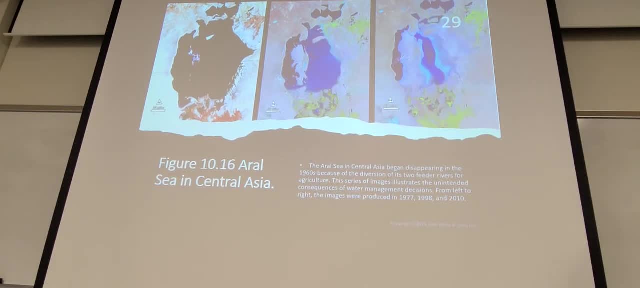 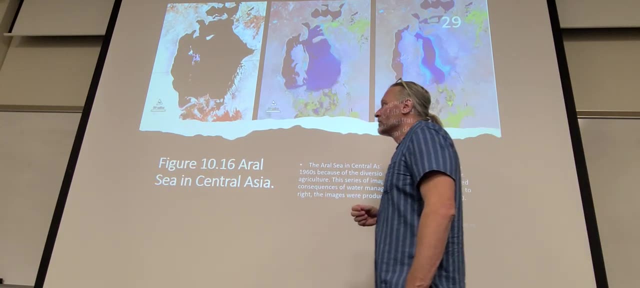 They should have corrected the color before they put this in the book. But what are you going to do? So there are a number of rivers that used to feed this body of water, And when those rivers were cut off for irrigation in different areas, then of course it started drying up And this is like a huge, huge lake, If you can imagine, one of the Great Lakes drying up. There was some attempts, when Russia was doing a bit better economically, to try to restore it And kind of, a little bit of it came back for a little bit of time. 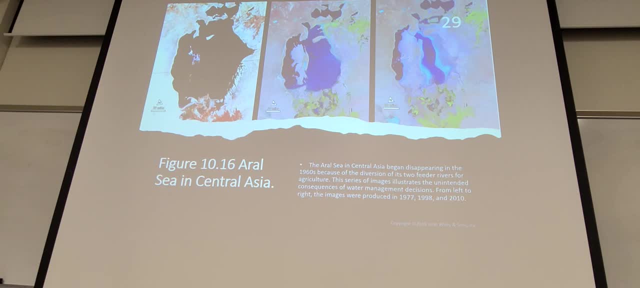 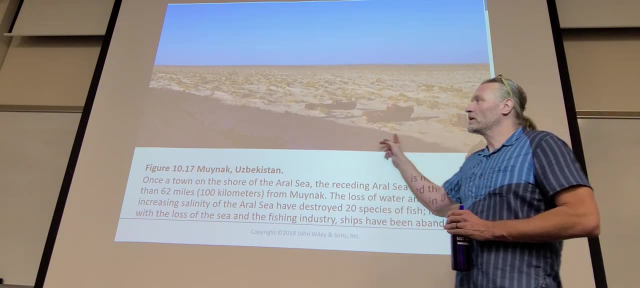 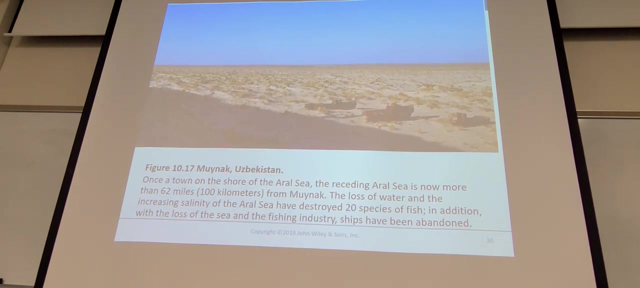 But then it quickly vanished again. But if you'll see news stories and stuff about this, you'll see these ships that look like they're in the middle of a desert right, Because it's a dry region. The whole region is dry. Without rivers feeding in. well, there's no water And what was there? quickly evaporated. Kazakhstan has, as I mentioned, there's a bunch of nuclear testing in the region, Somewhat similar to when the United States was looking at nuclear weapons before. 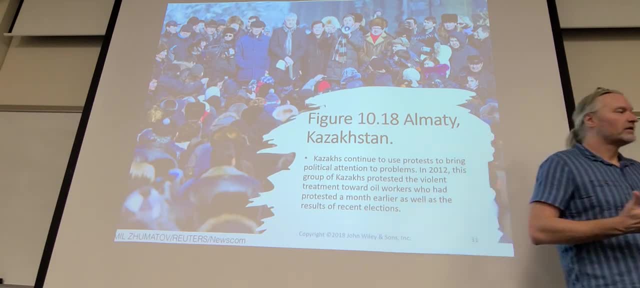 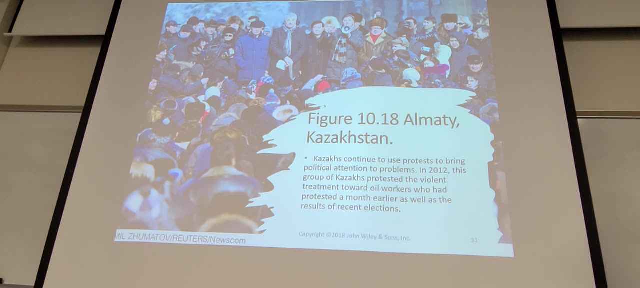 well, during the Second World War There's a lot of testing in Nevada, Because Kazakhstan was kind of their Nevada, Except for they didn't make an effort to make sure they were at places that didn't have people living, And so a lot of people got radiation sickness. 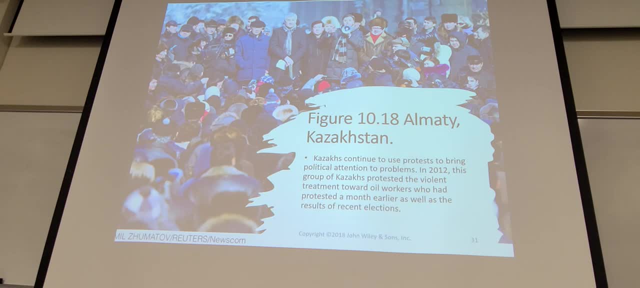 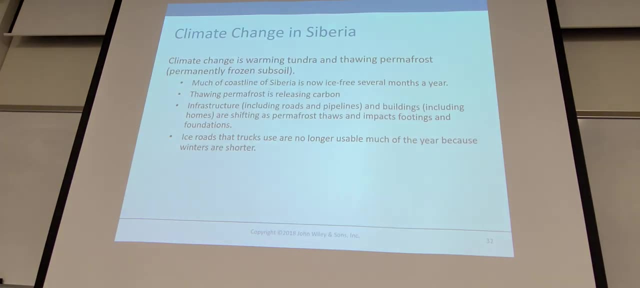 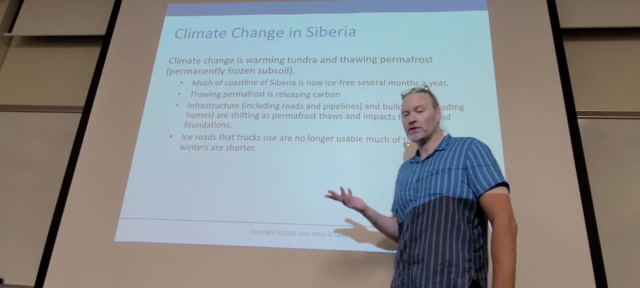 They didn't know what was happening. The Russians didn't let people know because they were keeping it all secret, right? I already mentioned a little bit about climate change in the far north. It's kind of interesting because, well, when it comes to 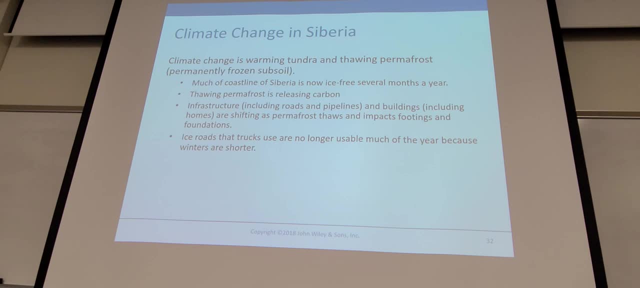 winners and losers when it comes to climate change. people in Russia are not really as against climate change as a lot of other places, Not just because it's a cold place. but let's see if I can get you back to the map. 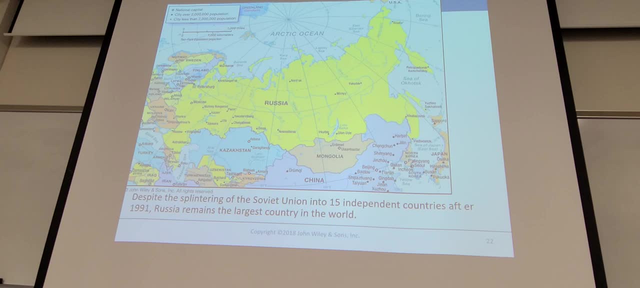 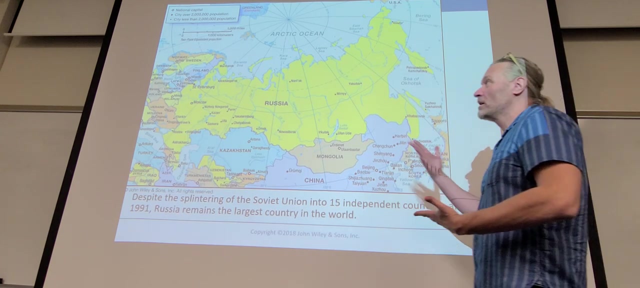 actually real quick. Russia, You can see they have a huge coastline, technically right along the north, But it is frozen in ice for a good percentage of the year, But lately it's becoming ice free for longer amounts of time, So it's a big shortcut for shipping. 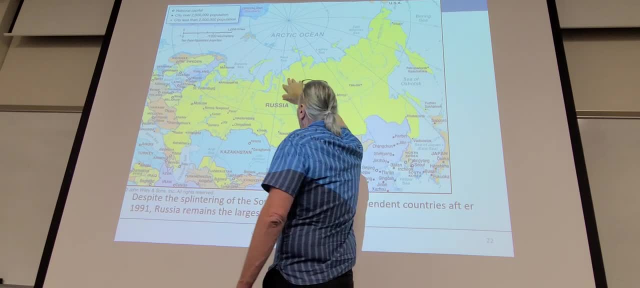 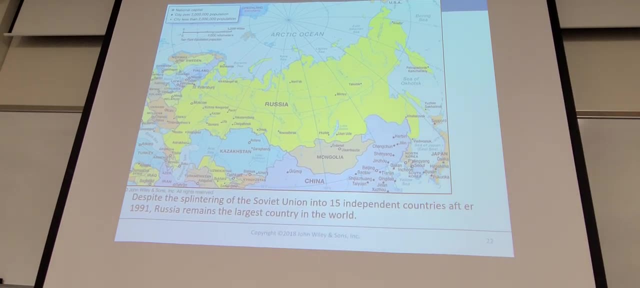 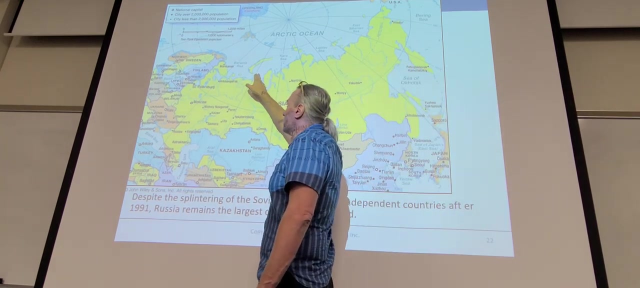 But also because there's all those natural resources up here, it's less expensive to ship it out. So that's been like one of the things that Russia has been okay with, And Russia has even started doing undersea ceremonies where they plant a Russian flag. 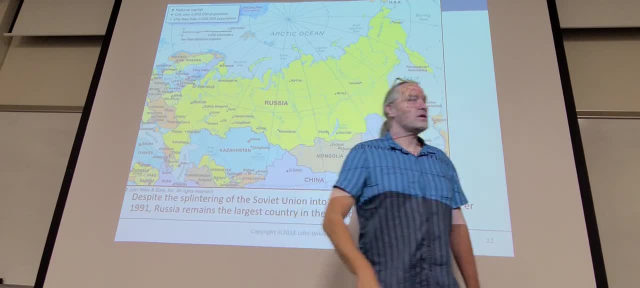 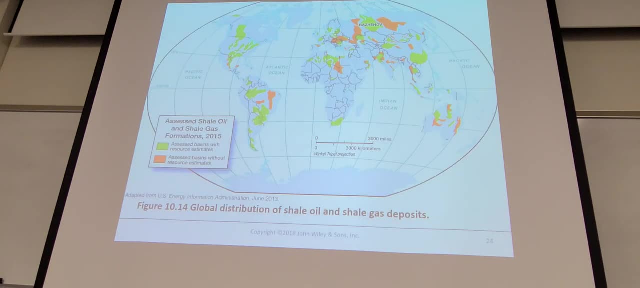 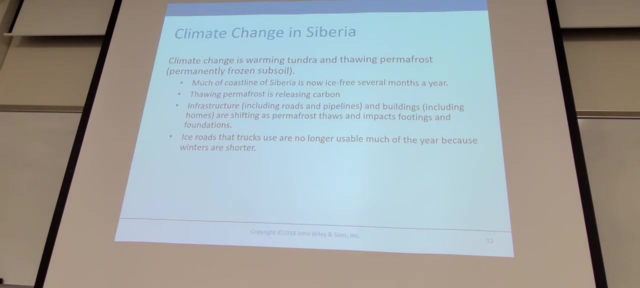 and start kind of saying which territories are theirs because they're thinking that there's going to be long-term resources in this region, Mining and things like that. Alright, going back to where we were, Let's see what else Permafrost right. 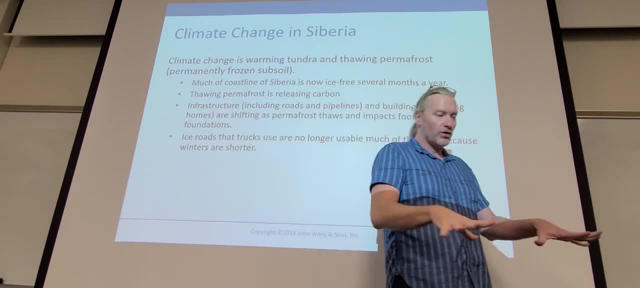 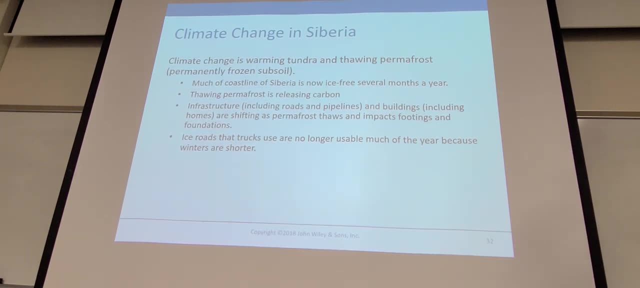 This is areas that, although the ground will thaw out and you'll get some grass and whatnot growing, there are areas under the ground that are permafrost, that are frozen year-round. Lots of those areas are thawing out And, if you'll see on the news, 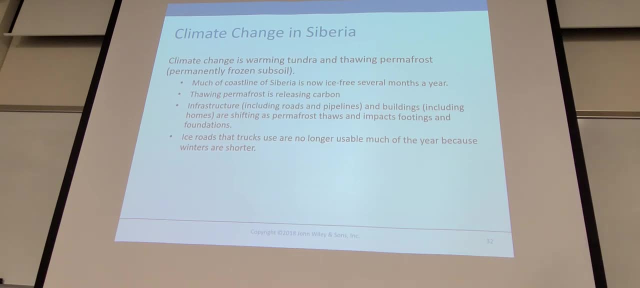 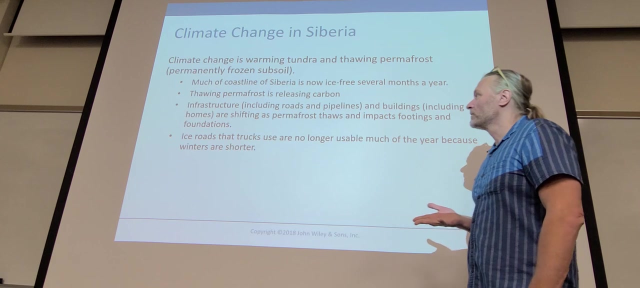 sometimes these giant sinkholes appear in places. That's part of what's going on there. It's also causing, like mudslides and a lot of kind of instability in the land. It also releases a lot of carbon. when this thaws out, Let's see. 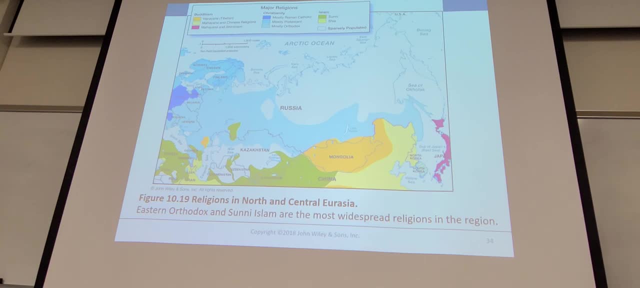 Religions in the region. Well, you know it's interesting because, well, it was Russian Orthodox. but then when the communists took over and the state ideology was specifically atheist, and this was primarily because they saw the church as a rival power. 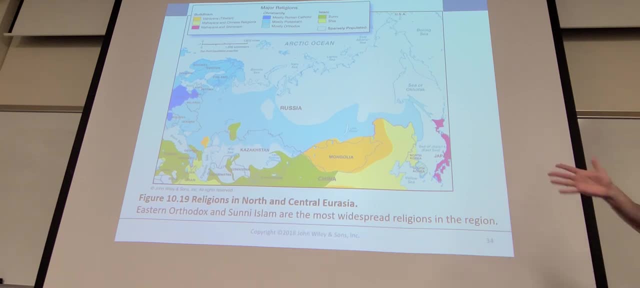 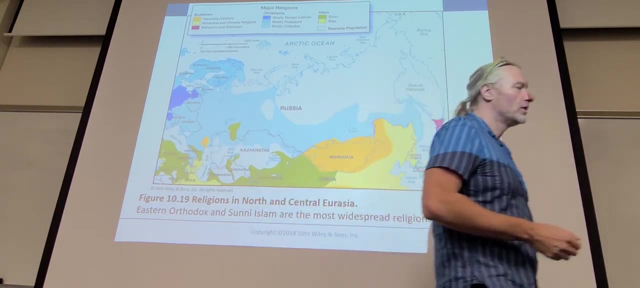 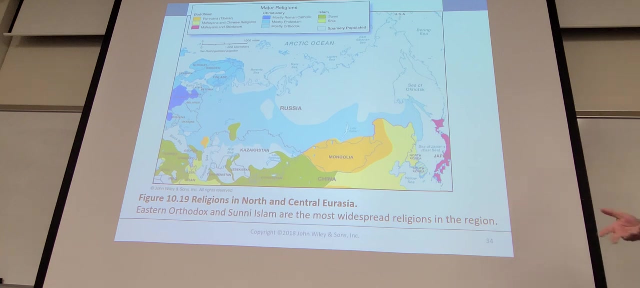 And so they- well, they wanted the churches to be gone. Since the Soviet Union fell, there's been a bunch of people coming back to religion, sometimes coming back to languages that had been repressed, coming back to customs and things that had been lost through time. Interestingly, although the Russian Orthodox Church was very much persecuted, the countries that were in this area that are mostly Islamic, they were allowed to still practice their religion. but Russia did have specific connections to the leaders of the different religious sects, basically had their loyalty. 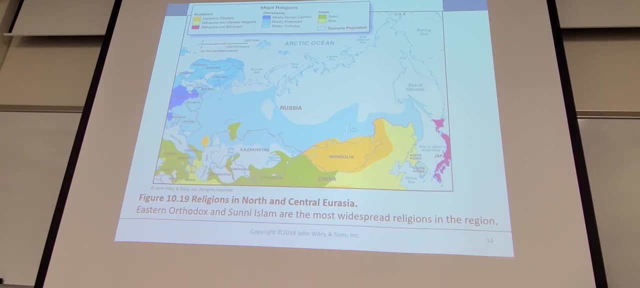 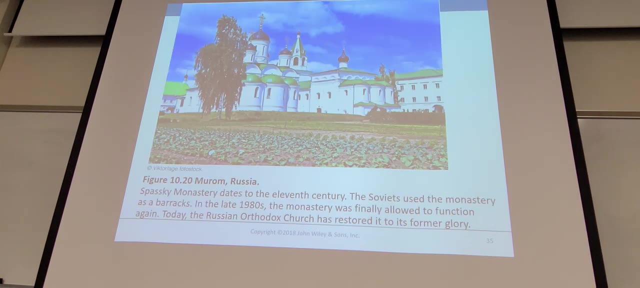 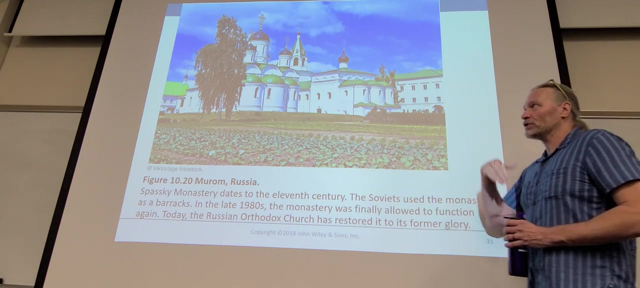 But that was a bit of an unusual thing for Congress, A bit of an unusual thing for communist countries to do to allow a religion to kind of stay. A lot of these religious buildings during the Soviet era they were changed over to other things. 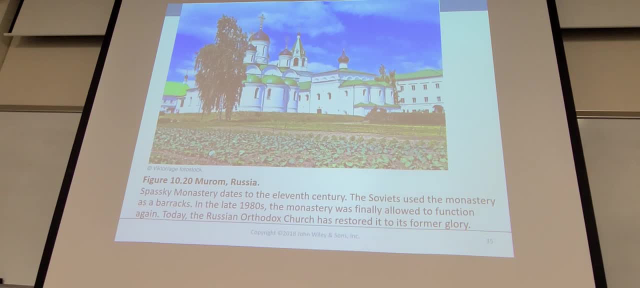 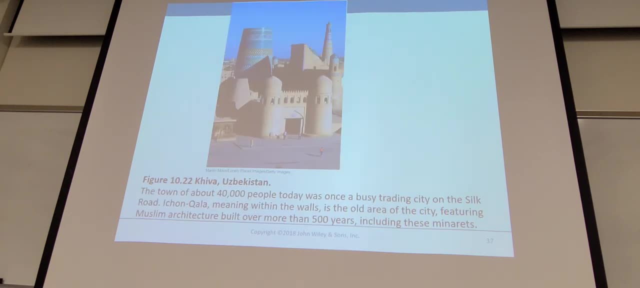 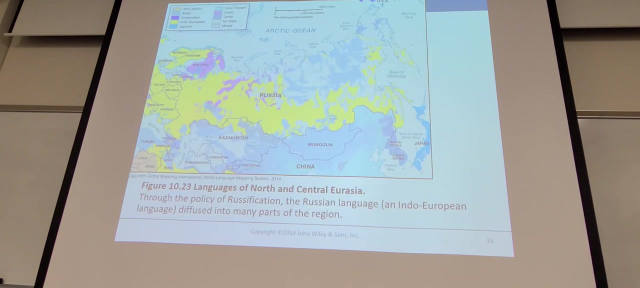 and now they've been kind of brought back sometimes Languages in the region. let's go to a map. Well, the map doesn't tell you a lot because it's just. this is that general Indo-European map. You can see that in areas that are more what we call Siberia, 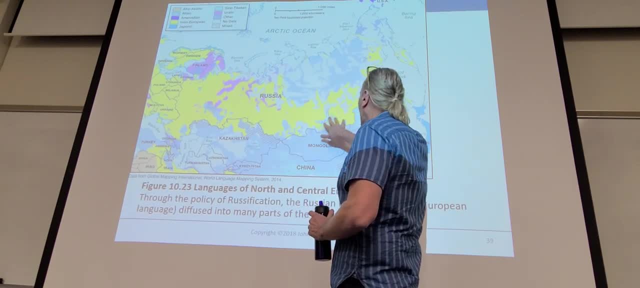 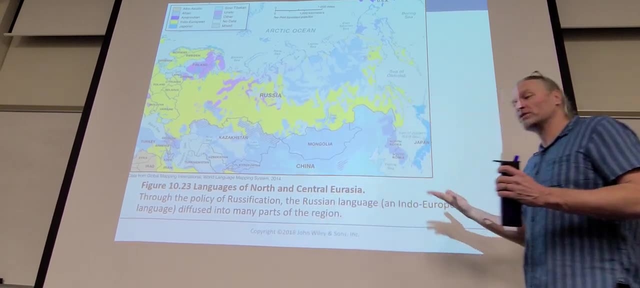 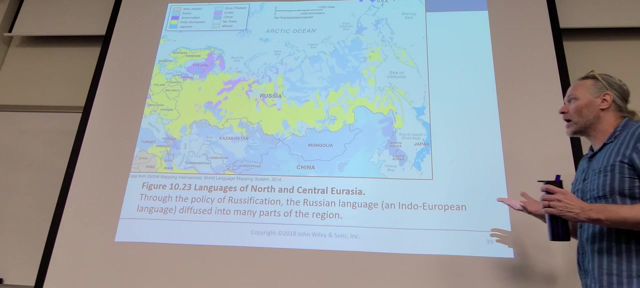 we have some different languages and again, the populations that are along here. these are populations that were shipped out, mostly when Stalin was in charge and he was shipping people out to Gulags. People have heard about that kind of thing Probably in Russia before. A lot of these populations when the Soviet Union fell and they were able to move back. a lot of them did, but a lot of them didn't, Because they were second, third generation people and now these places were their homes. 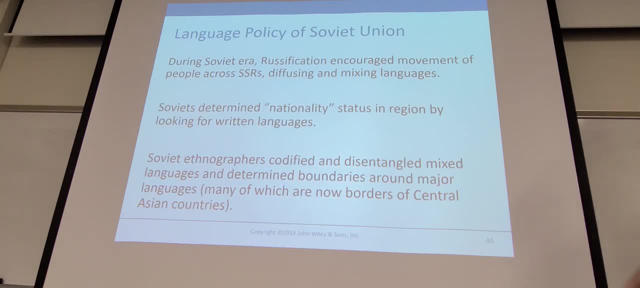 I also talked about Russification a lot. Just a reminder: Russification, what that meant. Although they talked about it being one unified Soviet Union, it was really Russia, and within Russia, Moscow, that was determining the policies. Joseph Stalin. 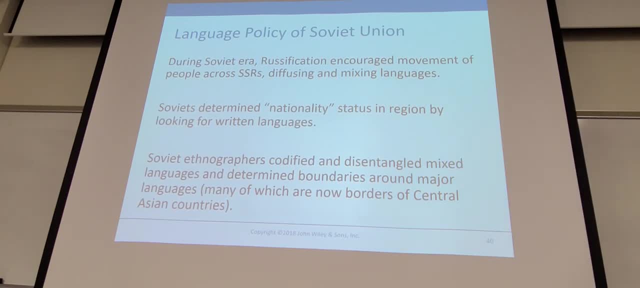 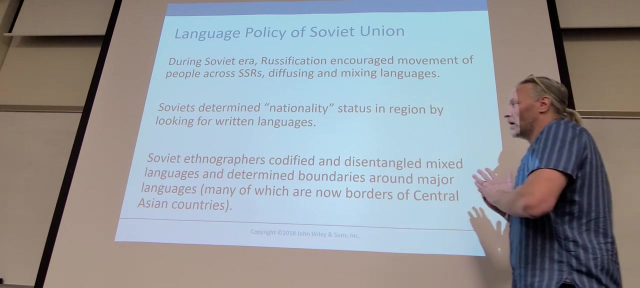 specifically when he got into power, which was just a couple years after their revolution. Lenin was the main person who was leading the Bolshevik revolution, but he died of mysterious causes shortly after and Stalin moved in. Stalin was very much in the old. 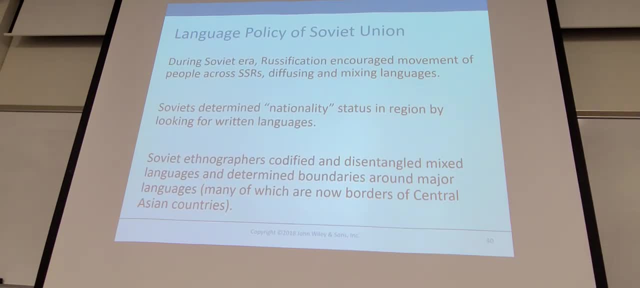 very imperial kind of way of ruling, and he personally felt that his culture, well the Russian culture, was superior to the other cultures that were in the other Soviet republics, and so everybody should be taught- not just Russian- the language. 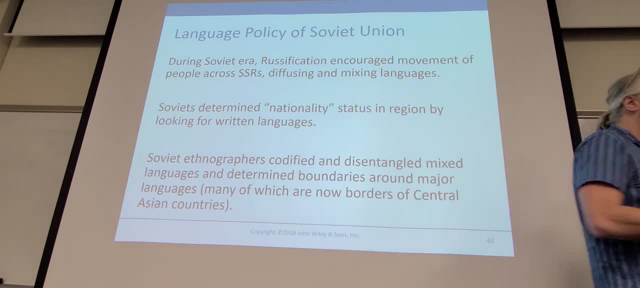 but all the kind of cultural norms, and his plan was that well that the other places would become assimilated eventually. And even though it's, you know, the Soviet Union is long past, it's a long history- the Russian language is still a bit of a. 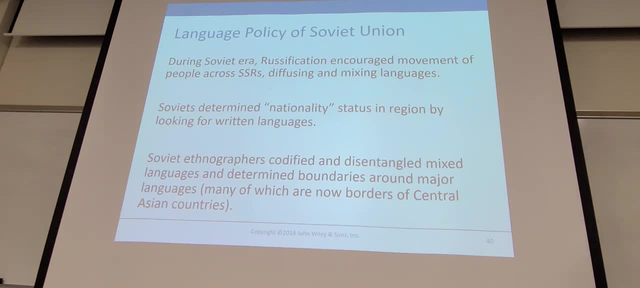 lingua franca in the area where people use it to communicate with each other, or in different areas. Yeah, Didn't the leaders of the Soviet Union occupy Iran's capital, Tehran? There's still some Soviet influence there, When I don't know, but like I was reading. 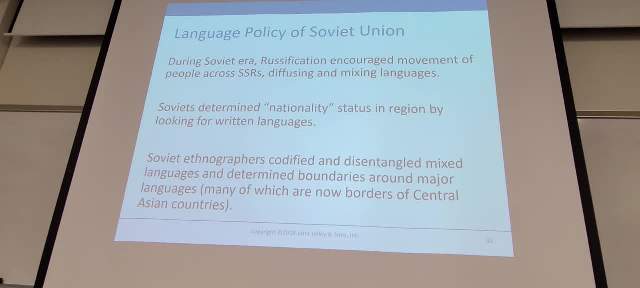 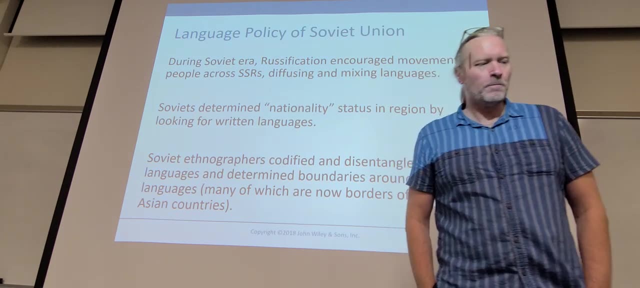 the last ambassador of Iran to the US died recently and like there was articles I was reading about the Soviet influence on Iran during that time. Like architecture government, I could be wrong completely, but I'm not sure. 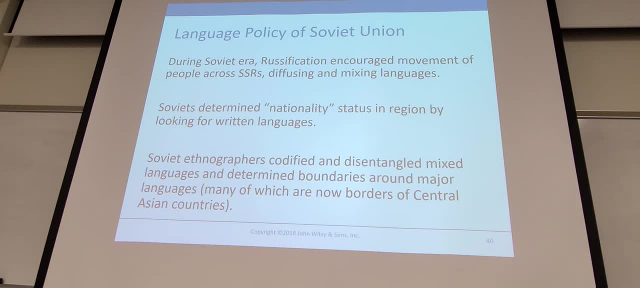 Well, I mean, the Soviet Union definitely wanted to have influence in Iran. I don't know how strong it really was- Me neither, Maybe before the Iranian Revolution, but I don't think anymore though. No, All right, Keeping on. 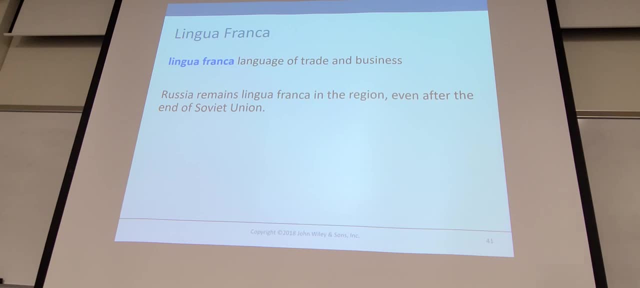 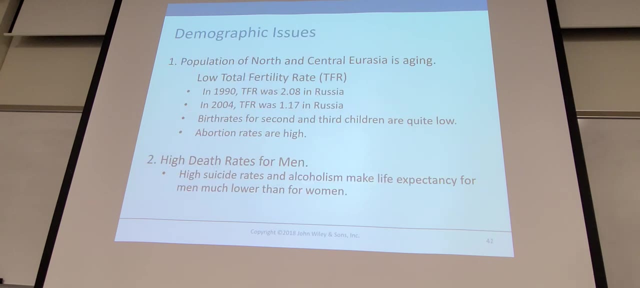 Oh, I just used the term lingua franca, language of trade and business. Very often it's English. today, in much of the world Demographics, We talked about how lots of places have falling populations because they have falling birth weights, right, 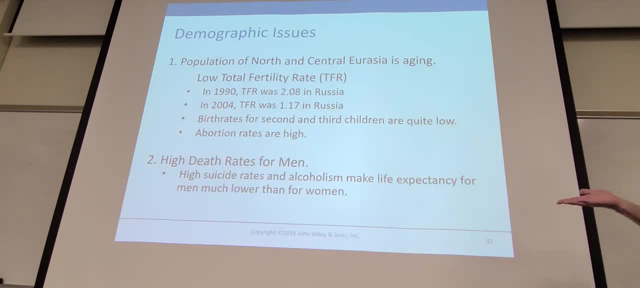 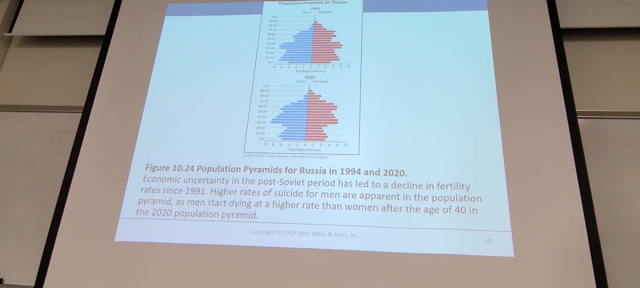 Russia. this is more interesting and more intensified than lots of other places, especially because you have higher death rates for men due to alcoholism and suicide rates. Let's see, do we have a population pyramid? So the population pyramid. you see a couple different things. 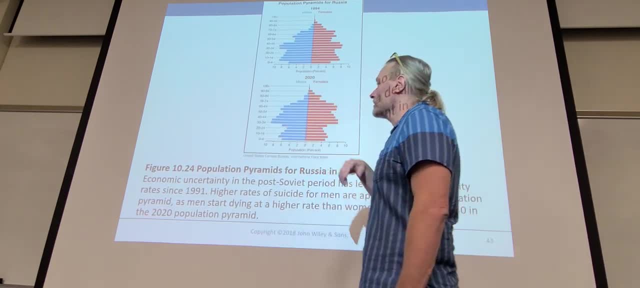 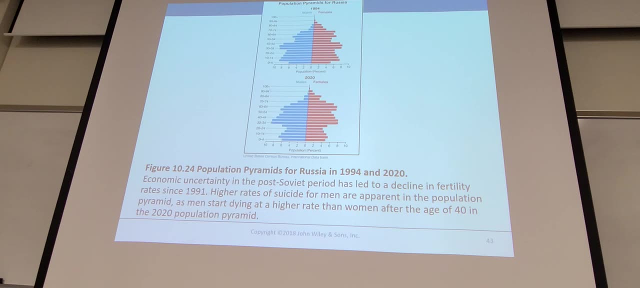 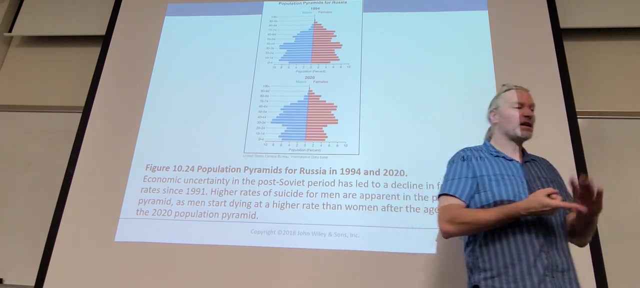 But one you could see. well, less males, right, And that's because of this high death rate- Living living well, I would say. after the Soviet Union fell especially, it was such a period of instability, People stopped having kids. 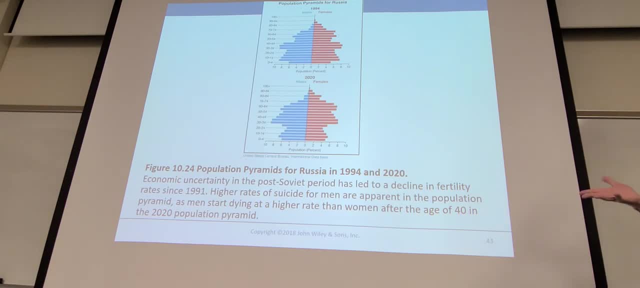 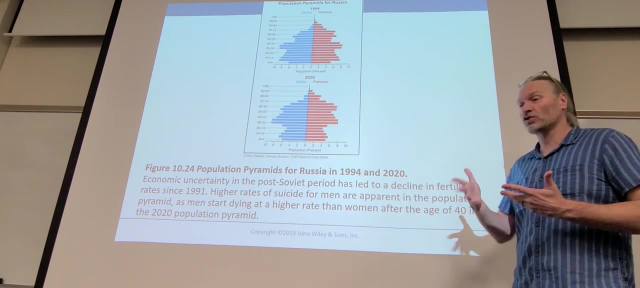 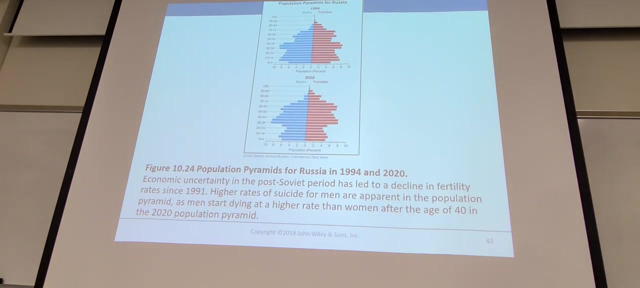 because people were very worried about their future. A lot of people felt hopeless, turned to alcoholism and other things, turned to suicide And their society is still kind of dealing with the effects of that. But I mean, what it does mean is 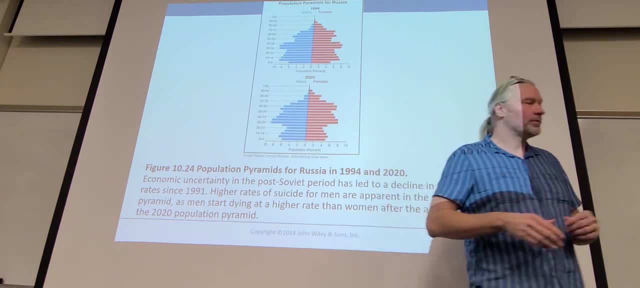 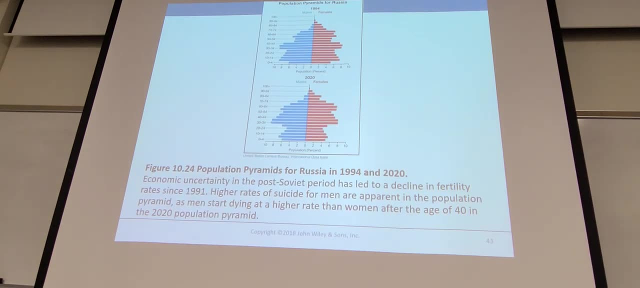 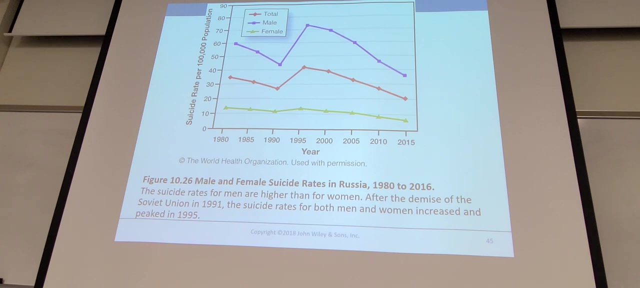 you don't have a population pyramid that's inverted so much As you see in other European countries, But it's not the best way to have that population equaled out generationally. Male and female suicide rates: As you can see, these really went up. 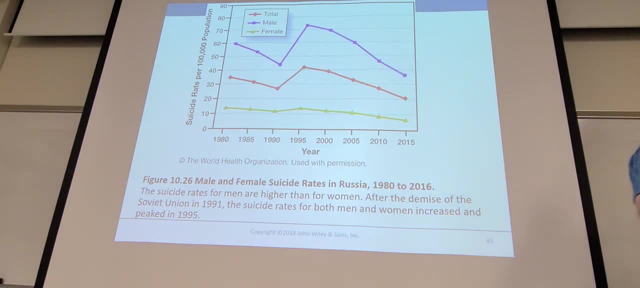 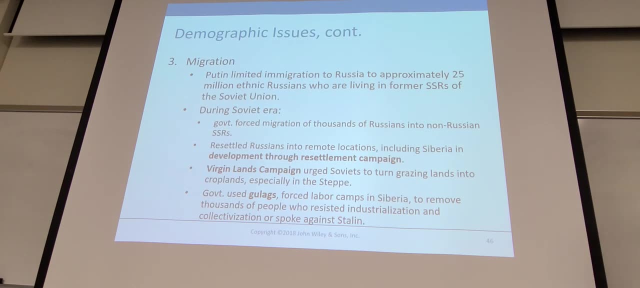 right after the fall of the Soviet Union And have changed somewhat through time. Other demographic issues: Not a lot of people migrate to Russia. Russia, when it comes to population not having kids, have a high death rate. for men, That means you have a population that's declining. Russia for a while. after the Soviet Union fell, they were allowing populations to move back. as I said, And although a lot of people moved back, it was still not enough to make up for the deficit of how many people have been lost through time. 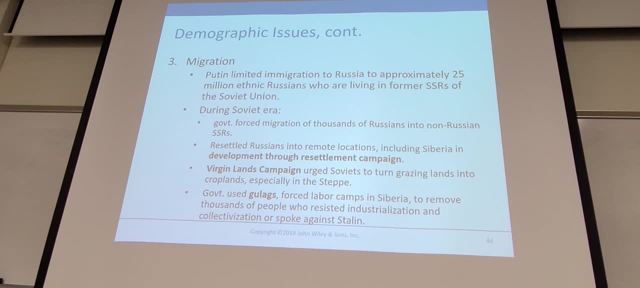 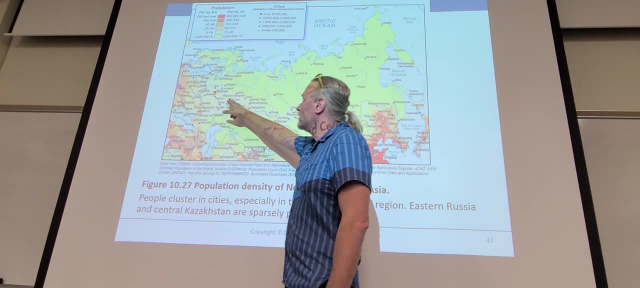 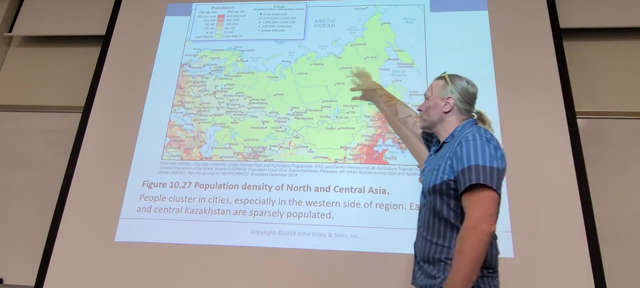 So in general the area has a declining population Population density. As you can see, the densest area might be around Moscow here, But when you get to the Ural Mountains it really really kind of not to say there isn't people here. 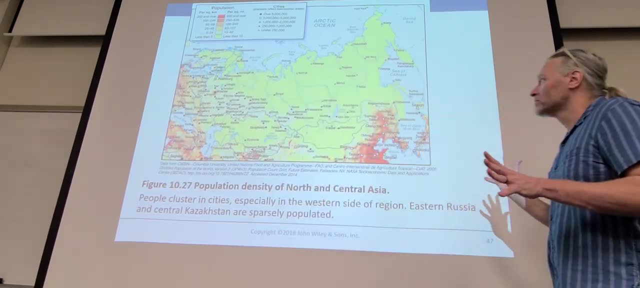 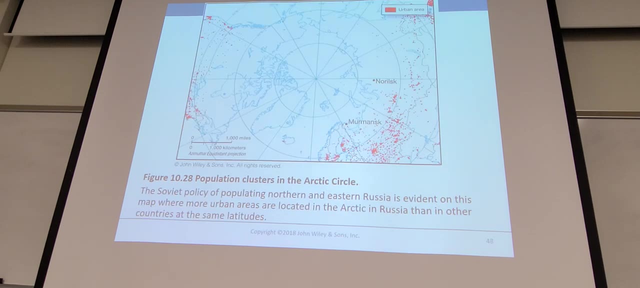 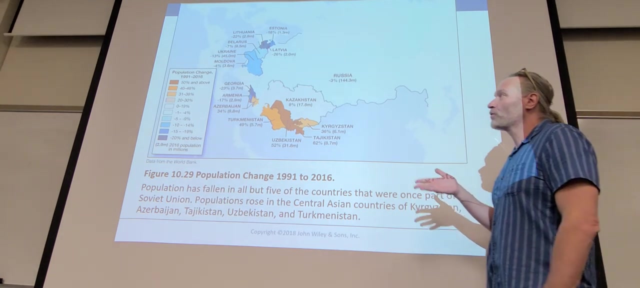 because there are cities and there are people, but it's very spread out And low concentrations. Looking at population change, you can see not all former Soviet republics are kind of in the same boat: right Places that are more on the Europe side. 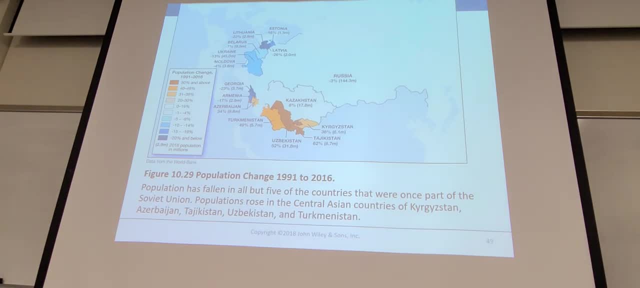 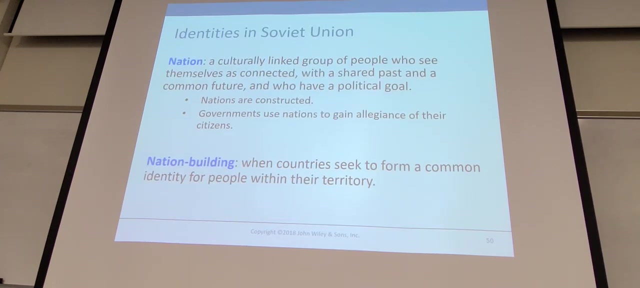 are kind of more similar to what's going on in the rest of Europe, But places down here more in Asia, having higher population increases, higher number of births. So let's see, During the Russification process, Russia was working on nation building, right? 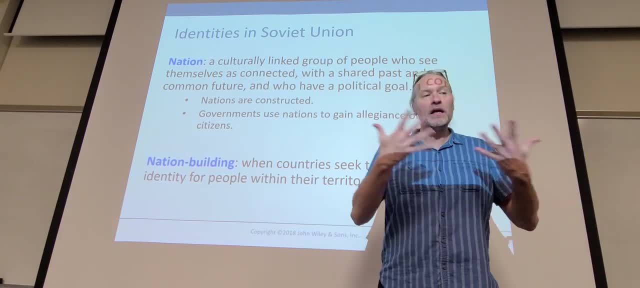 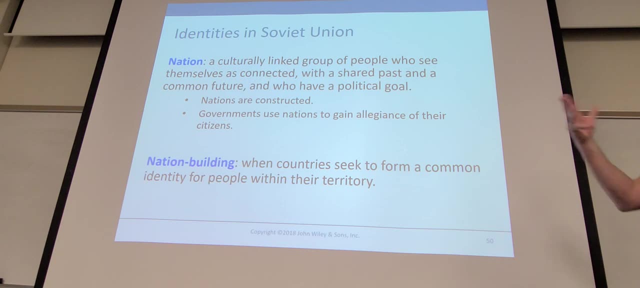 It was hoping that, by basically making everyone assimilate to this common identity, this Russian identity, that it would forge this larger kind of mega-sized nation right. Not what happened? It happened some, but not to the level that Russia had planned out. 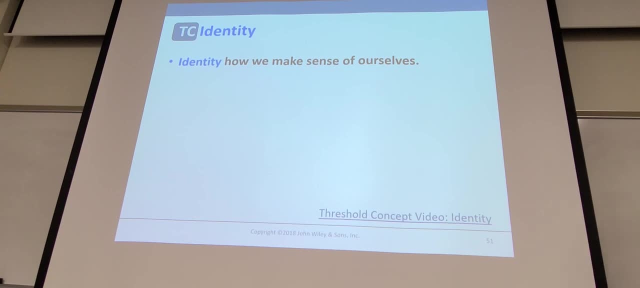 You know this is a term that we've actually used a lot in the book, but it comes up in this chapter as a term: identity, how we make sense of ourselves, Identity- it can mean a lot of different things In the context of this chapter. 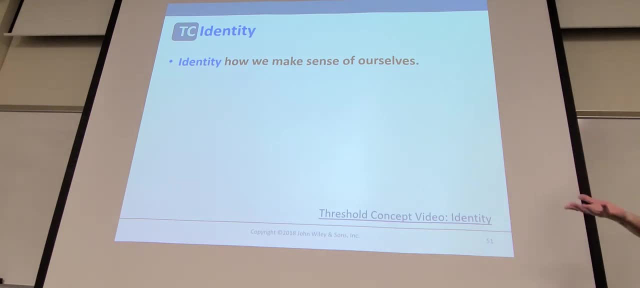 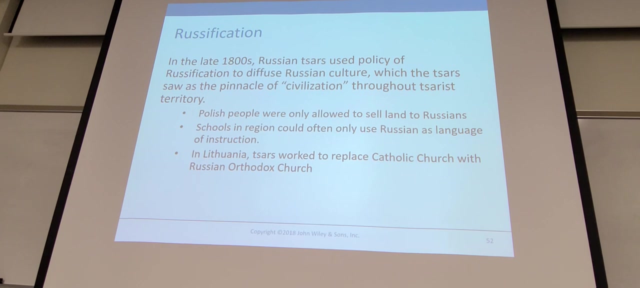 they're talking about national identity, right. People have different amounts that they feel tied up with their nation and that identity. Of course there's all kinds of identity, right? There's political identity and gender identity. All right, Russification. I already talked about Russification quite a bit. I should say that before the Soviet Union became a thing, before it was communist, it was the Tsars, which is just another name for royalty. The Tsars were cousins to the royalty of the other. 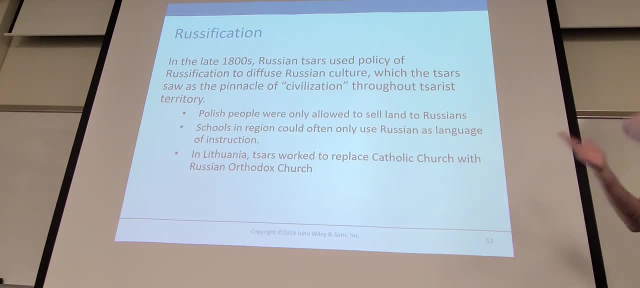 European countries. In fact, if you look pictures of them side by side, they would look up and they looked almost identical to the other royal families. It was kind of a lot of inbreeding among royal families in Europe. Well, during the Tsars, 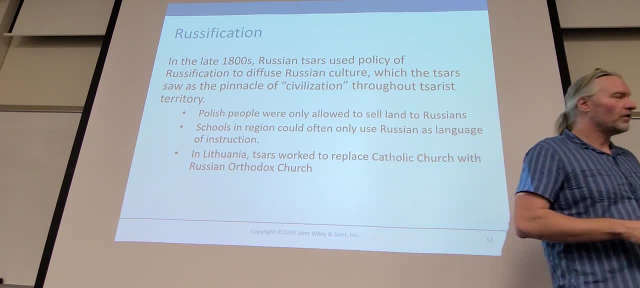 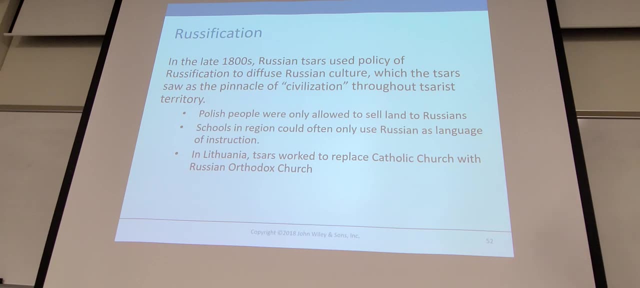 they were also trying Russification. They were doing the same thing. So when they had control of Poland, they made laws so that Polish people could only sell land to Russians, right? So the Russians would slowly kind of take over Teaching Russian. replacing the Catholic Church with the Russian Orthodox Church. Again, this was during the Tsar period of time. So when the, when they had the communist revolution, lots of other countries in Europe had revolutions against their monarchies. This was similar to that. There were some differences. When the communists took over, they killed the royal family, So there wouldn't be any risk of them coming back to power. Um, Let's see. Actually, most of this stuff I've already talked about. Um. 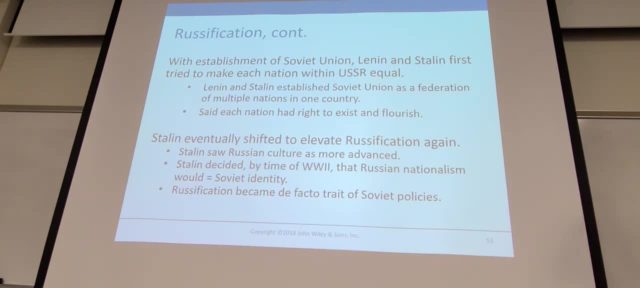 I will just say, though, that when the the kindness revolution happened, it was against the Tsars, it was against the monarchies, similar to other places in Europe, Um, But in Russia, well, you had that same thing, where you had a bunch of people who moved to the cities, and the cities were full of people. They were overpopulated, A lot of people were very, very poor And um the businesses there, whereas in the rest of Europe a number of people had become somewhat prosperous. Um, In Russia at this point in time there was still mostly a lot of people who were very poverty-stricken And people saw the royalty and capitalists as kind of in the same boat, as people who had all the resources and weren't given any. 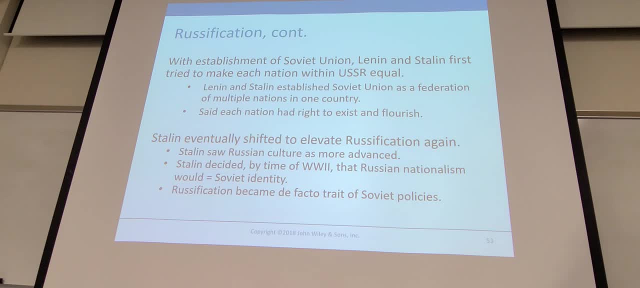 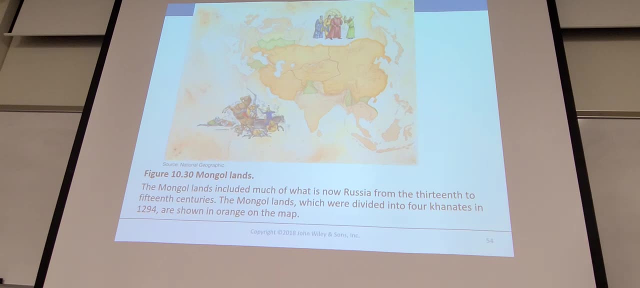 Um, So this is, this is part of why there's a popular uprising there, as well as other communist places that were going through a similar thing. Um, There's a little bit in this chapter just reminding us that, uh, this land. 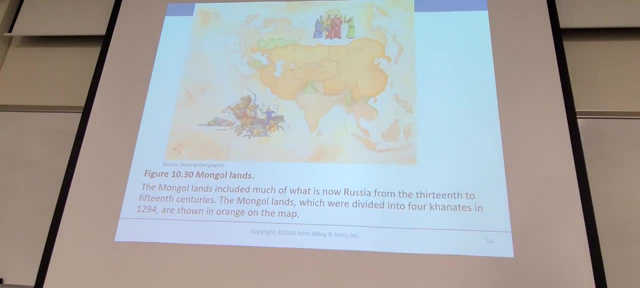 before the Russians was uh, under control by, uh, Mongolia, right, This is part of the larger Mongolian Empire way back when, Um, And they did. I guess it would be called Mongolization, Um, Having people learn their language, their customs. 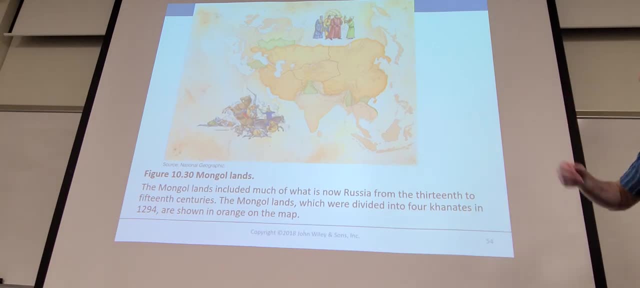 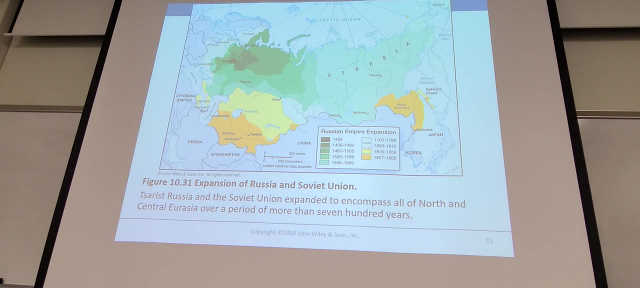 This is one of the reasons why when people think of Russia, they think of it as a place that's kind of a mix between Europe and Asia. Um, Because it's had these cultures kind of in charge at different points in time. Now the Russian 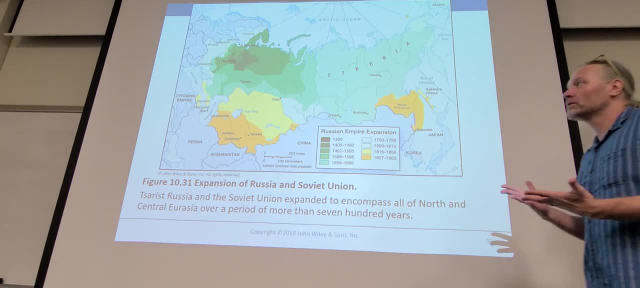 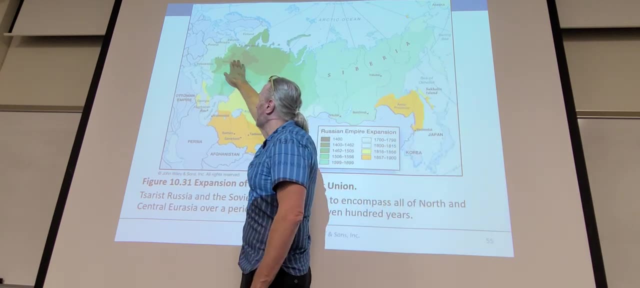 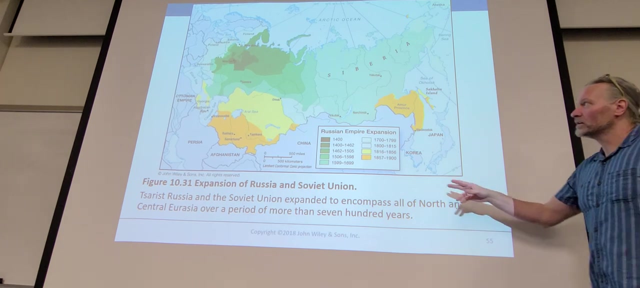 the Russian Empire, the Russian people. um, It was well, as you can see, they started from an extremely small hearth right, Extremely small area and, through time, expanded, expanded, expanded, and you can see this expansion was before. 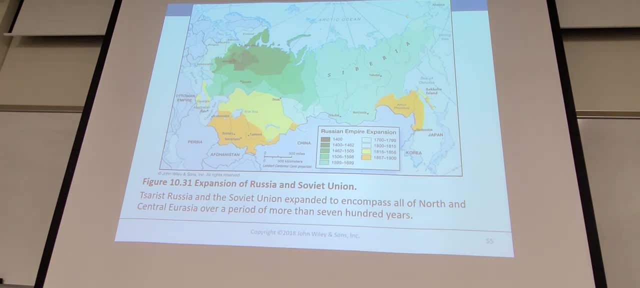 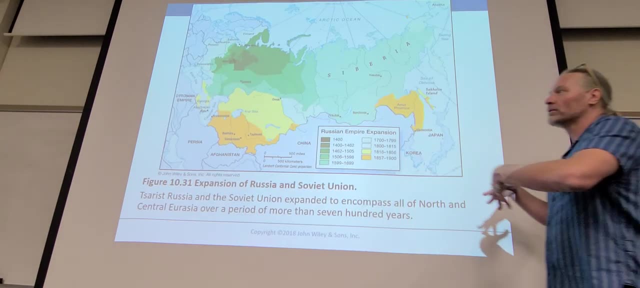 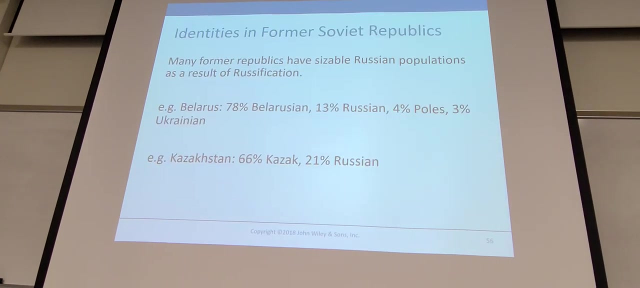 the communist time right. Large expansion to these different areas. Mostly they're going into areas, especially after the Mongolian Empire kind of decayed. They just started taking places that had been controlled by them. Uh, Also part of Russification, moving Russian populations. into the different places, right? That's why a lot of these places have a significant percentage of population that are still Russian in those places, even though they were born there and they've been there for sometimes a couple generations. Um, This is why the questions 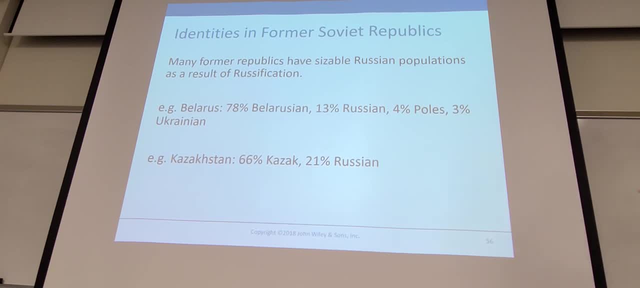 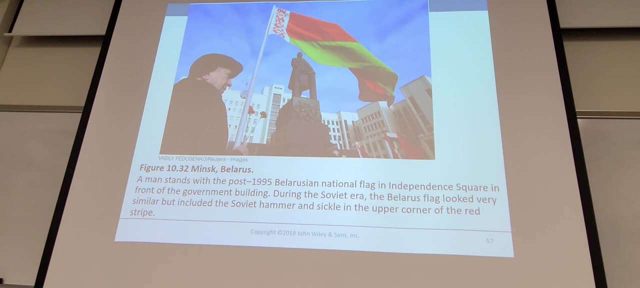 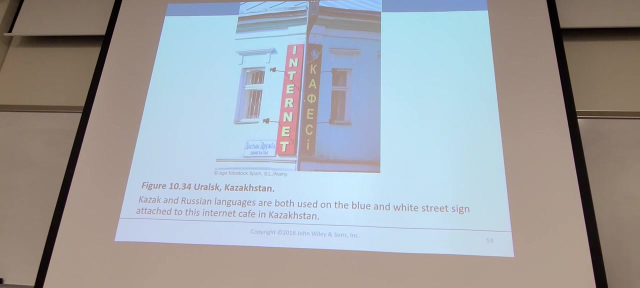 about well how Russian these places are. aren't as cut and dry as you might think. Uh, I don't know if people have ever been to Canada or countries where they have things in two languages. if you've been to Quebec, Um. 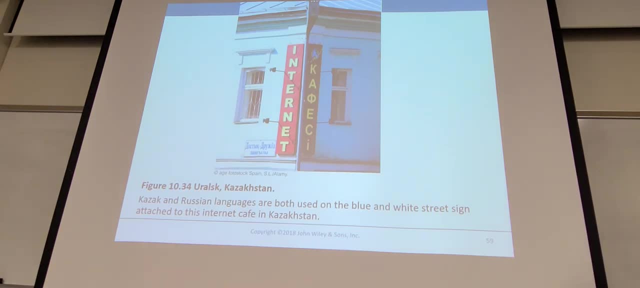 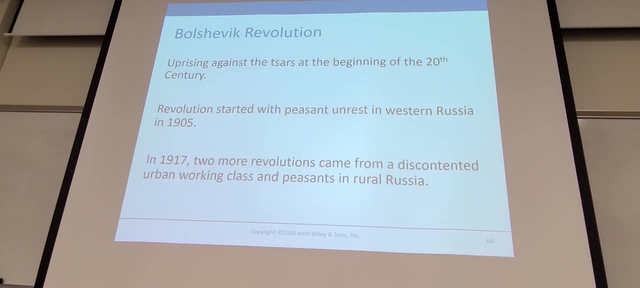 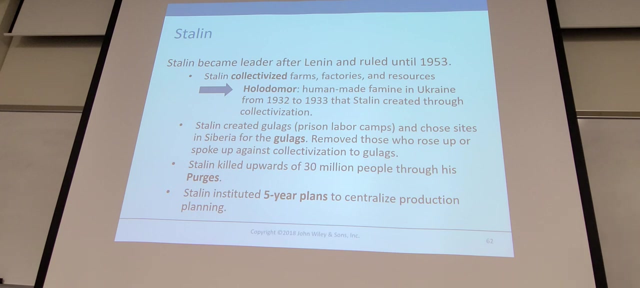 That was a thing often in many places, where they would have everything in Russian and then also in the local language. Um, Now I talk about the Bolshevik Revolution. Um Well, Talk about Stalin a little bit. Joseph Stalin, Um, That's not the name he was born with. He chose. Stalin means steel, And so it's as if you became a political figure and you're like my name's gonna be Joe Steel now, Because I'm that tough. That's what he did. He literally named himself Joseph Stalin. 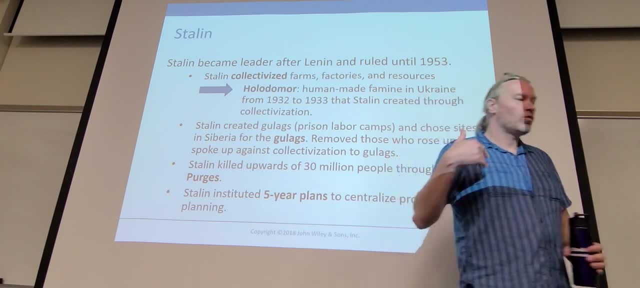 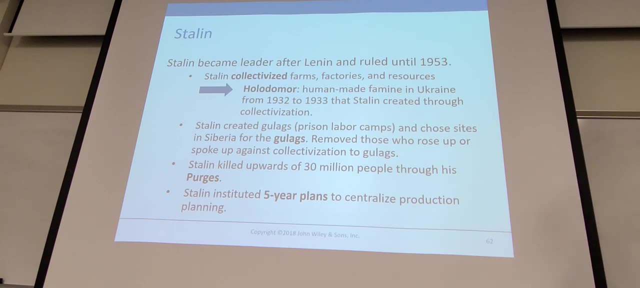 Um Well, When, When he came into power, Um, He started a lot of repression, Right Um An example: a huge famine in Ukraine, where the communists took all the agriculture that was produced, All of it, Uh, So locals. died. It was about one and a half million people starved to death Um Lots of different places that Stalin felt were not loyal enough. He would kind of put through mass starvation Um, And then places where the populations were smaller amounts that he felt 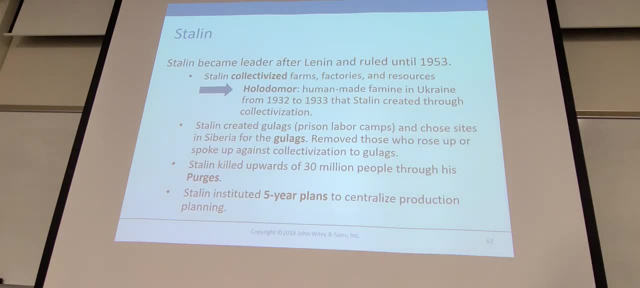 were not loyal to him. If he didn't have them killed off, which he often did, He'd have them sent out to gulags, And that's all along that border there. Uh, That he sent people out to, Um, It was very effective. 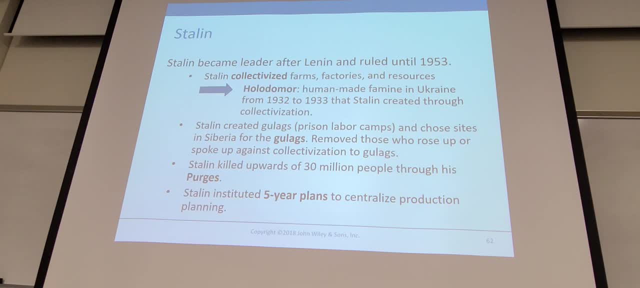 Uh, People were too terrified to really go against him. Um, But you could see upwards of 30 million people through his different purges. They call it different purges because it was a number of years that he had power and control. Uh, It's interesting because when he died. Russia went through a thing where they specifically tried to distance themselves from the things Stalin had done, Because none of the stuff had been kept secret. It got out to the whole world that he did these things. that killed a lot of people. 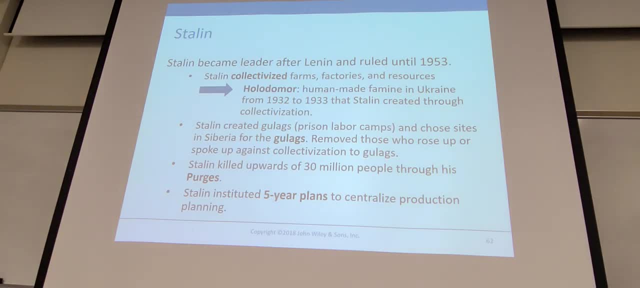 Um, So Grushenkov, who was, I think, the first leader after him who had been a big victorious general during the second world war, so he had a lot of power. Um, He specifically came out against Stalin and said the country needed to move beyond. 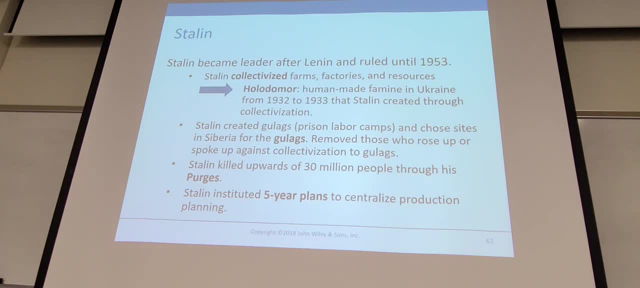 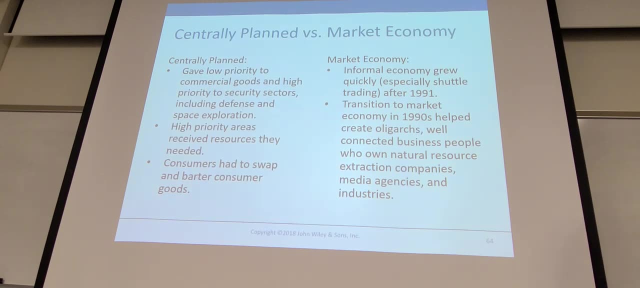 uh Stalinization. Centrally planned versus market economy, While this area had a centrally planned economy for many years. centrally planned economy means: well, your government decides what's going to be made and how much of the stuff is going to be made. 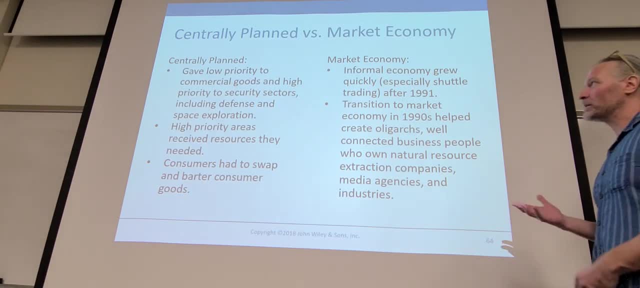 Right, It's not a supply and demand. Um, So what does that mean? In general, there is huge shortages of things, And so people would be in big lines, Uh, And also there was still demand for a lot of things, And so this is when. 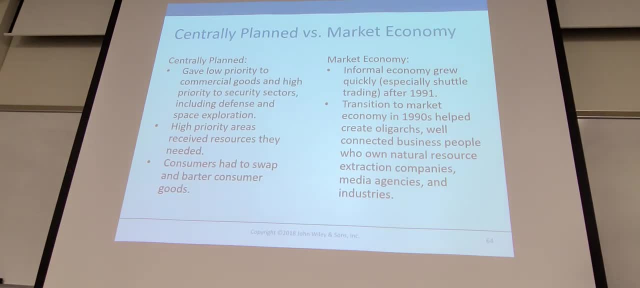 uh, smuggling in became a giant thing. Um, And the Russian, uh, the Russian mob, organized crime, Um, And today's Russian olgarks, many of them got their start uh, shuttling in things from, say, Turkey, Things just like blue jeans. 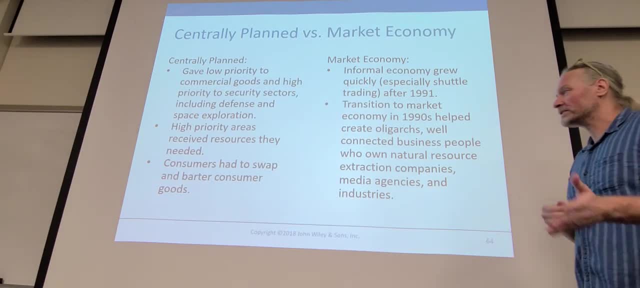 They would sell for a lot of money. Um, They would be bringing things in and obviously that was part of the underground economy, Um, But it was very prosperous. It was very wide spread, Uh Cause, again, there was huge demand for these consumers. 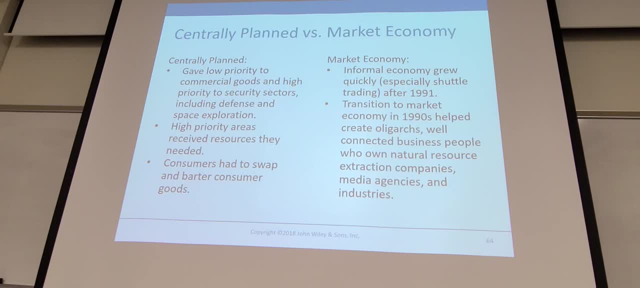 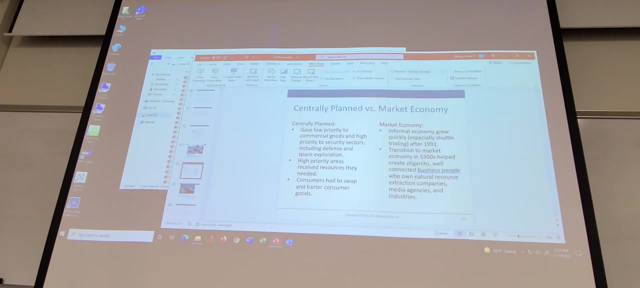 Uh, I've talked a good amount of time. I think I'm going to have you guys work on a couple questions. Let's see. Well, not a ton of time. Let's see What can I do. Let's see. 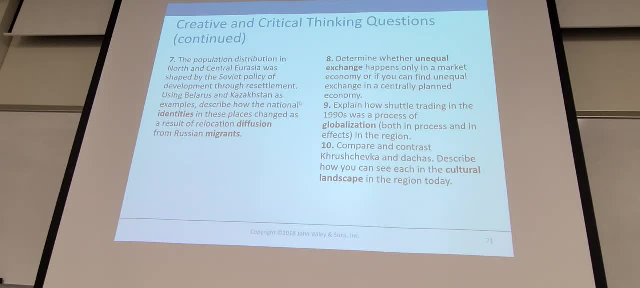 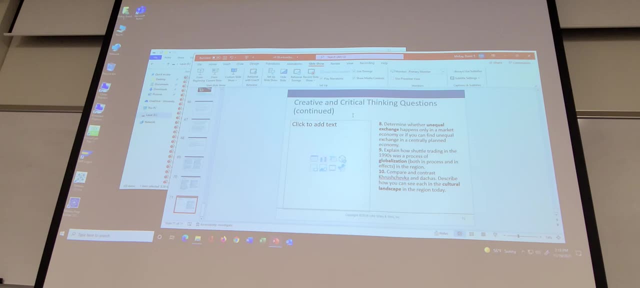 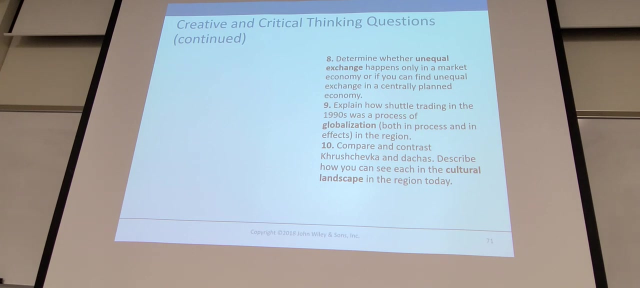 There's too many questions for most of you. Alright, I'm going to take off this one. I'm going to have you work on three questions. Let's see. I may have you self assemble into groups, Just because it takes too much time.